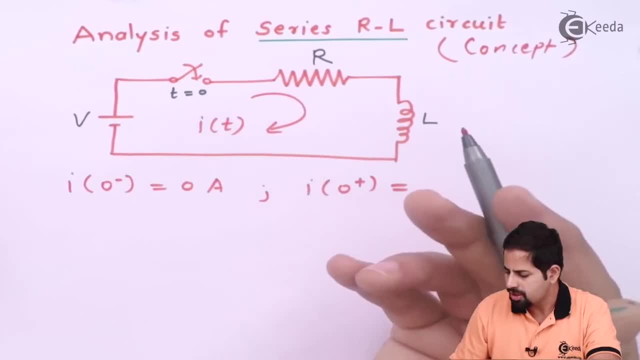 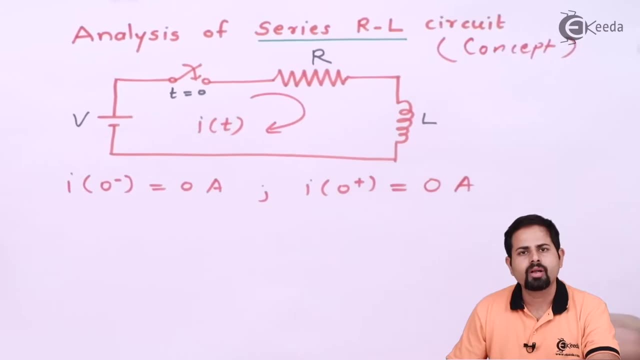 open circuit because it doesn't allow any sudden change, and so I of 0 plus when it acts as open circuit, it will be again 0 ampere. So here we have got I of 0 plus equal to 0 ampere. Now when I close the switch I can write the differential equation, So I of 0 plus is also. 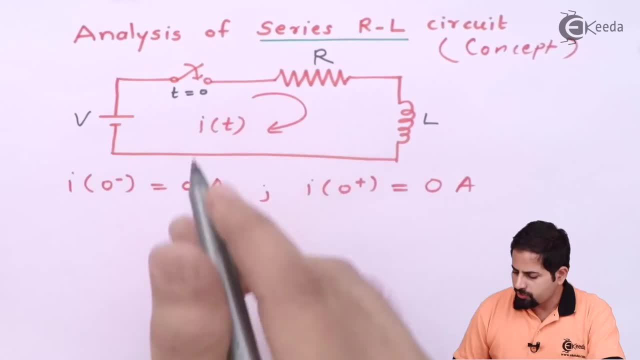 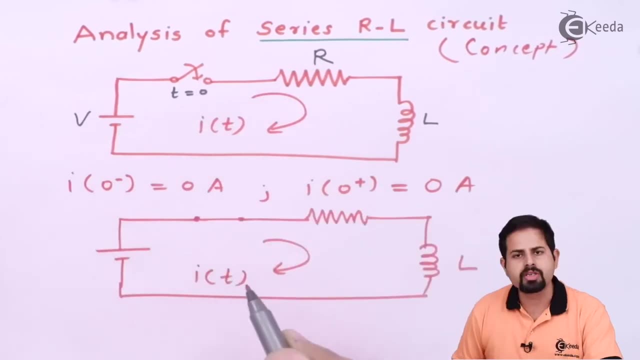 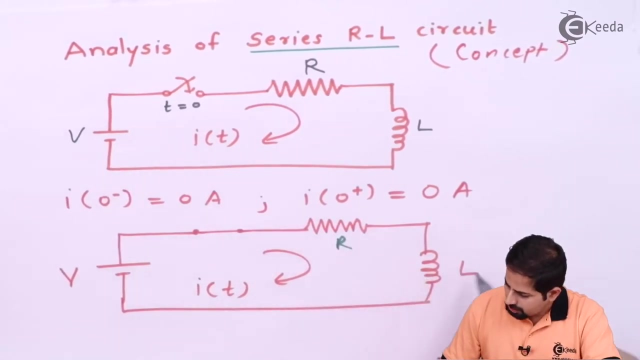 equal to 0 amperes. Now, when I close the switch, the circuit will become like this: This will be the voltage source. The switch is closed, So current, which is function of time, and here there is voltage source, and this is resistance R, This is inductance or inductor L. Well now, if I apply, 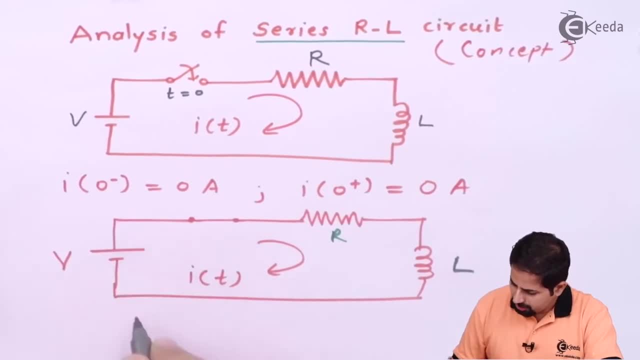 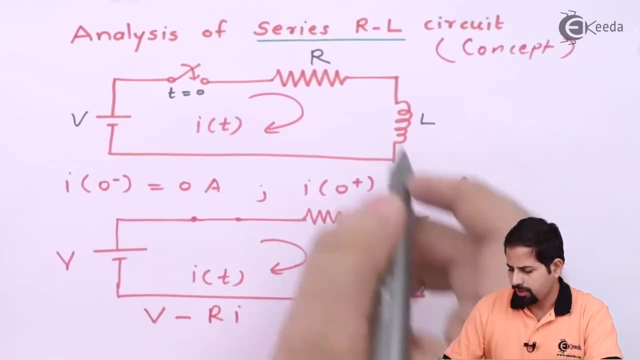 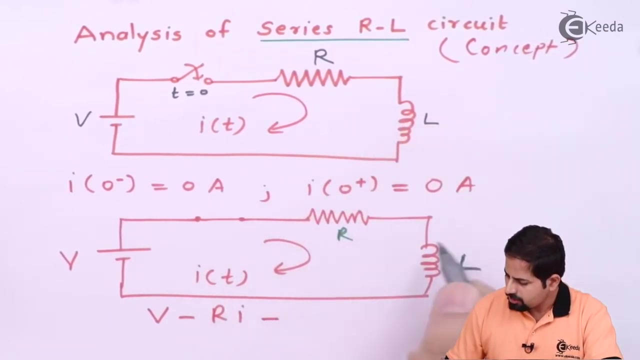 KVL to this. I will come to know that see V minus r into I. here I am not writing I of T T. It is assumed that throughout this analysis current and voltage are functions of time. So RI minus the voltage across inductor is L DI by dT equal to zero. 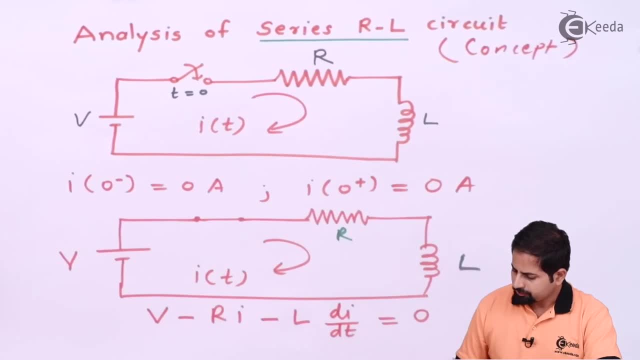 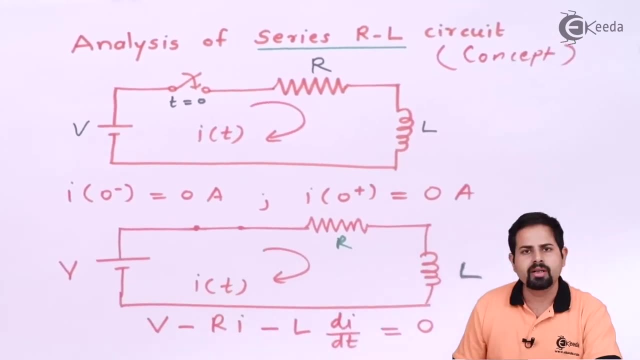 So now what we will do is- I will take these two terms to the right side. Well, there are two methods, but the second method we will see later. This first we will see the little bit difficult and lengthy method, because that is the basic method. So I will 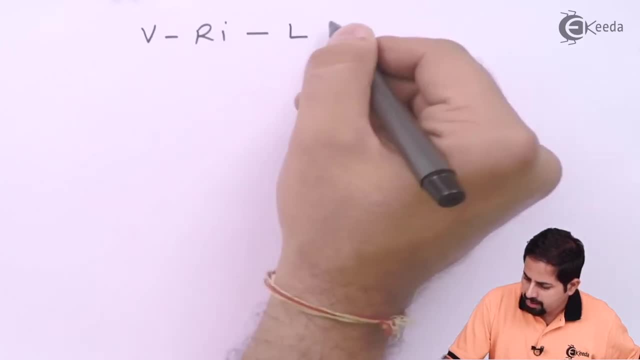 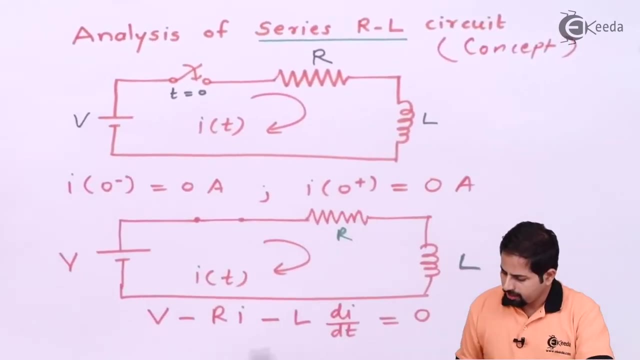 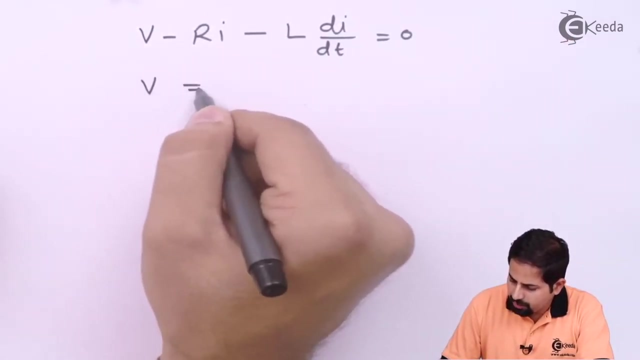 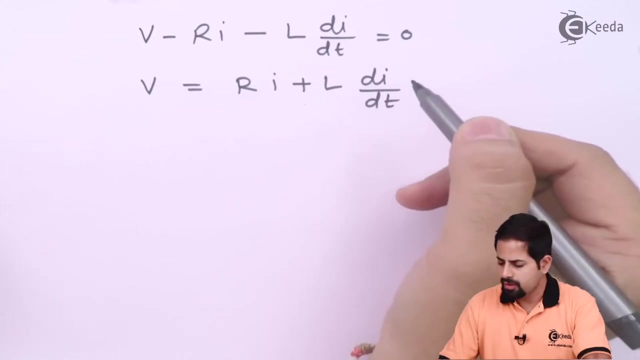 write the statement again: v minus ri minus l into di by dt equal to 0.. See the same statement I have written there: v minus ri minus l di by dt equal to 0.. Now here v is nothing but going to be ri plus l into di by dt. and so if I multiply by this: 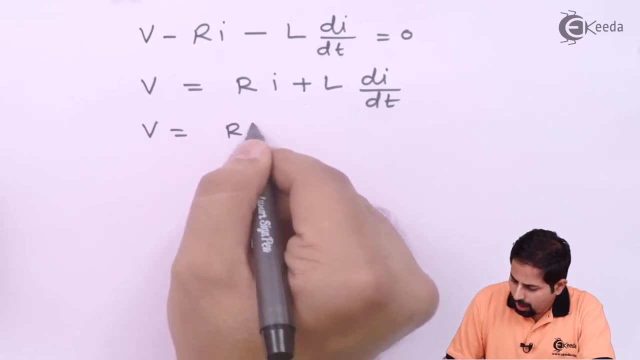 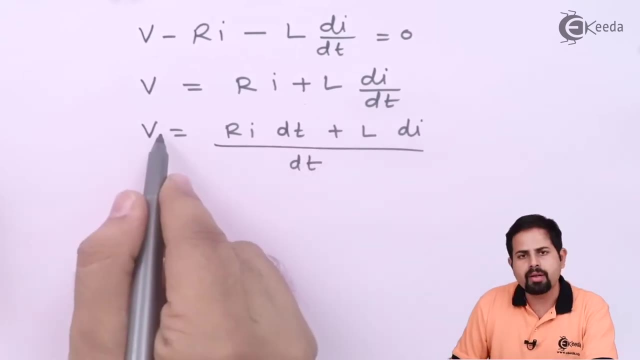 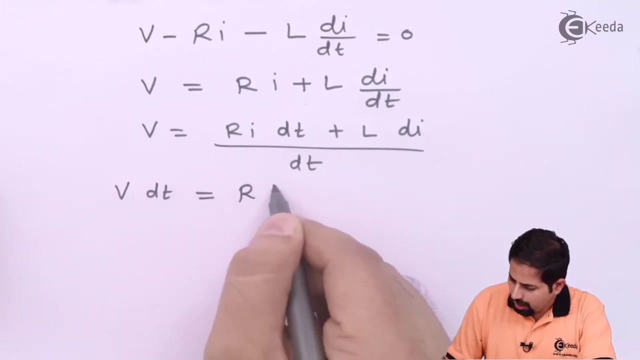 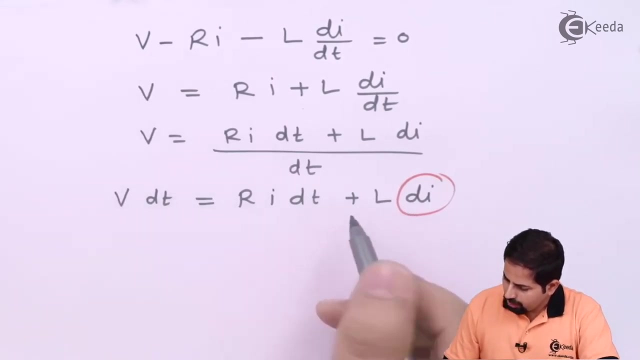 dt, I will get v equal to ri, dt plus l into di divided by dt. This dt I will take to LHS, So I will get v into dt equal to ri by dt. Now I want to find current, So I will leave this term as a solar term. So for that, what? 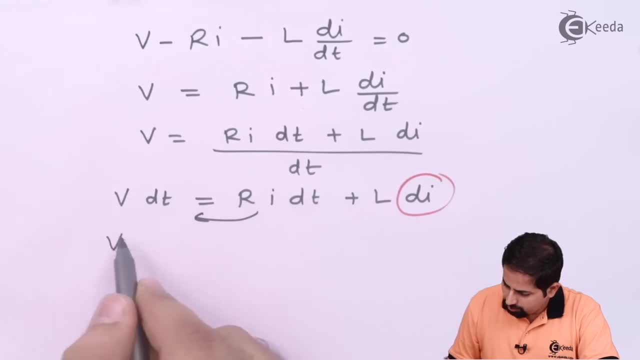 I will do. I will take this term to LHS. So I will get v minus ri in bracket because this dt and dt I will take common. I have taken this term, this term I have taken to LHS here. So v minus ri into dt is equal to l into di, or this term consists of current this one. 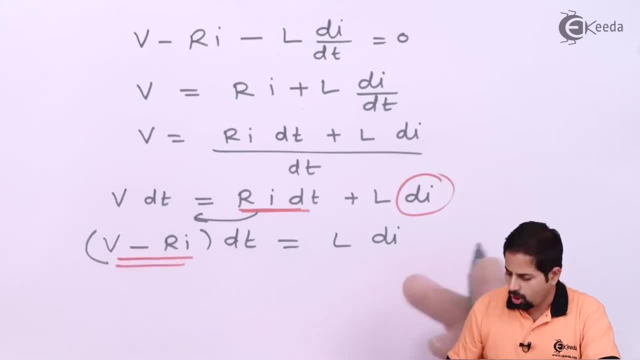 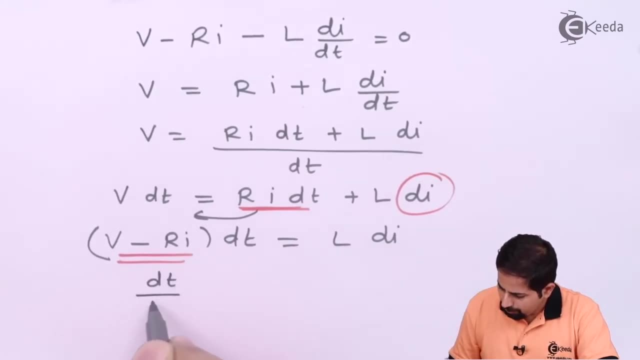 It consists of current, So this I will take here in denominator and this capital L I will take here in LHS. So I will get dt by l is equal to di upon v minus ri. Now why I have taken it in this form. for that we need to see the mathematics, which I will not see in detail. 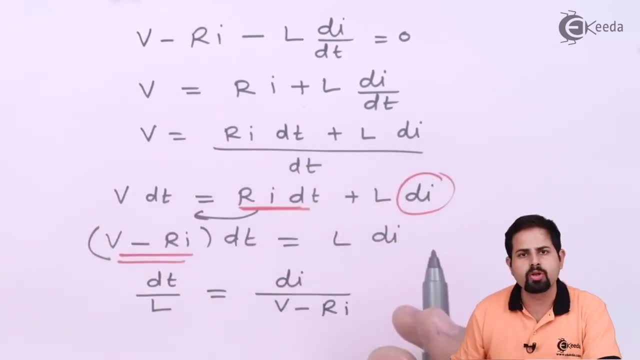 here, but the exact form of differentiation solution, of partial solution of differential equation, linear differential equations to be seen, and there is m, dx plus n, dy. that form and by those details we can get the solution. Now, if I want to get value of current I. 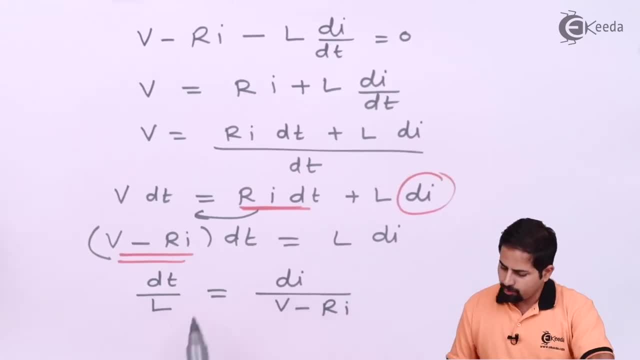 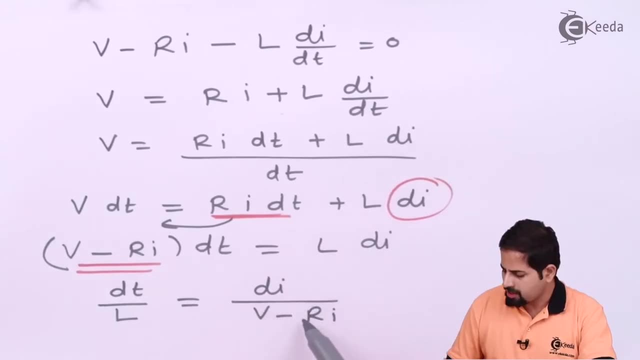 I will have to integrate both sides. So if I integrate here both sides, what I will get see here. So integration of this term will be: this is 1 by x form and integration of 1 by x is natural log x. So if you integrate this side, you will get natural log of v minus ri divided. 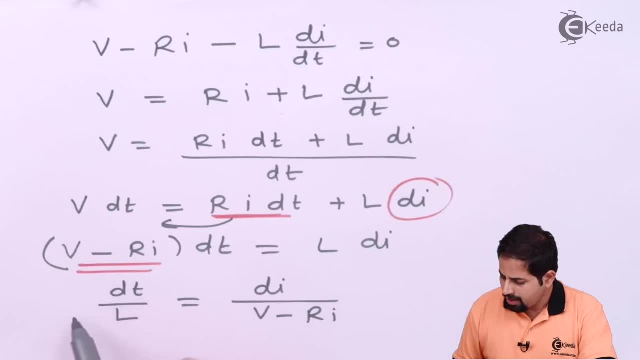 by coefficients of current, that is minus r. and here, if you take the integration, integration of dt will be simply equal to t plus the constant of integration. So I will write here and dt will this. 1 by l will be like this. So I will write here: and dt will be 1 by l will. 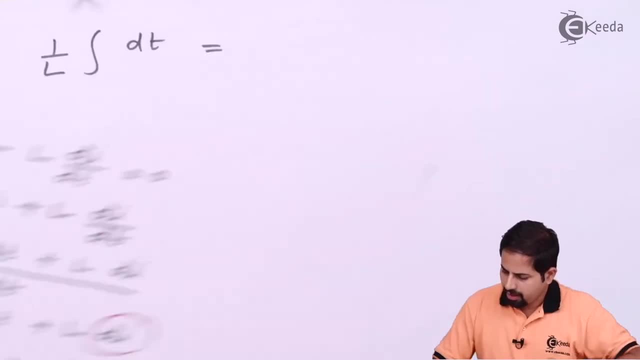 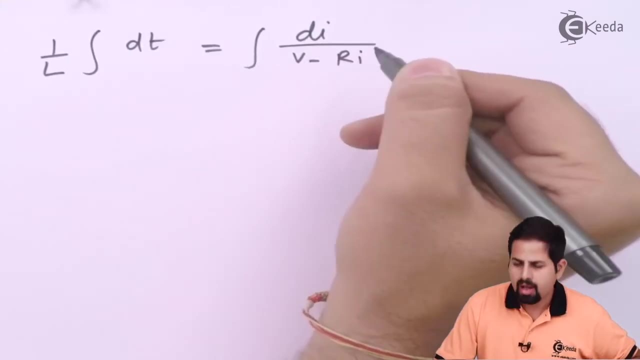 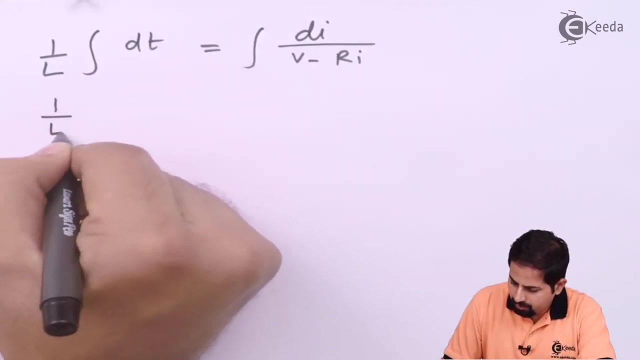 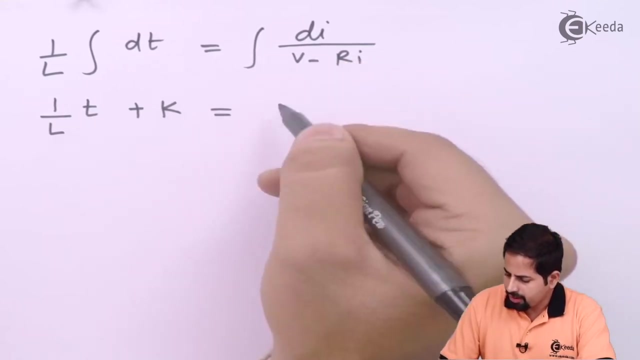 be like: this is equal to integration of di upon v minus ri. So if we integrate this we will get into t plus k. k is a constant of integration, and here I will get natural log of v minus ri divided by 0.. So I will write here: 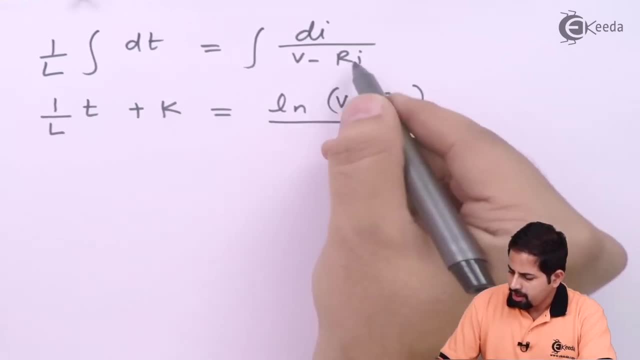 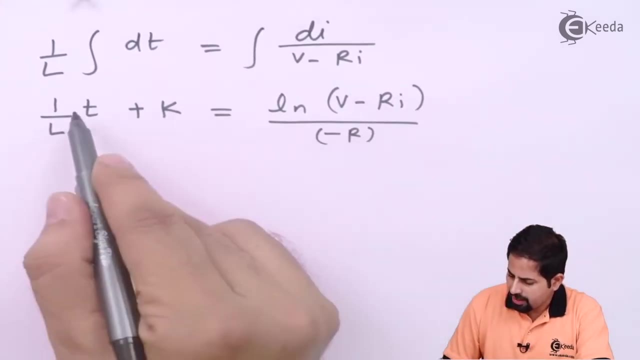 So I will write here. So I will write here. So that is the information about integration of. what we have is like this ER engine which is in the MI. Ok, Now I will take this: minus are here because I am interested in this term and see when. 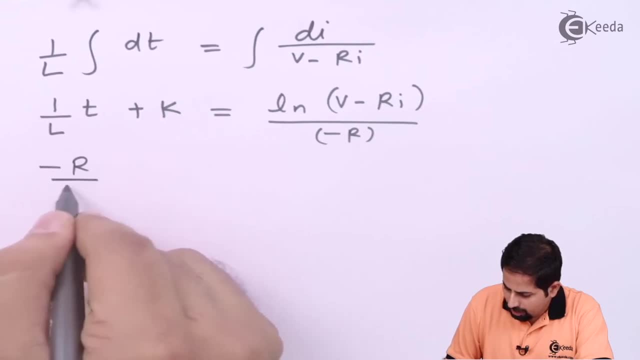 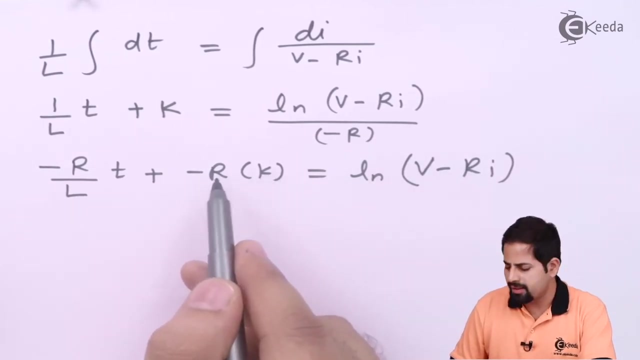 I take this, minus are here. it will become minus r upon l into t, plus minus r into k, equal to natural log of v minus ri. Now this is, k is a constant of integration. it is multiplied by minus r. r is a value of resistance, which is some constant. So we will say that their 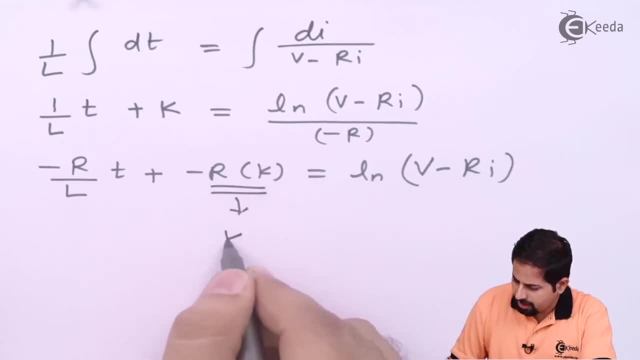 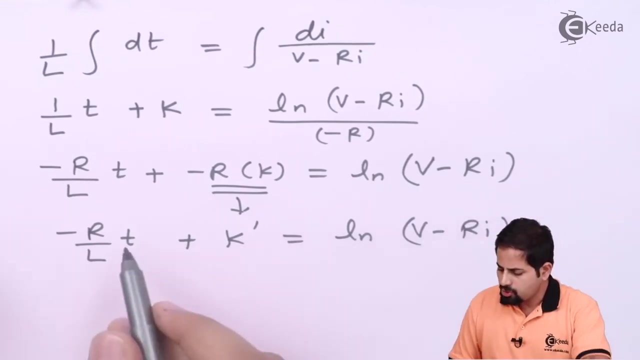 multiplication results in another constant called as k dash, and here I will have minus r by L into t, equal to natural log of V minus ri. Now if I want to solve this somehow, I need to introduce natural log on both sides so that I am equate terms. and so what I will? 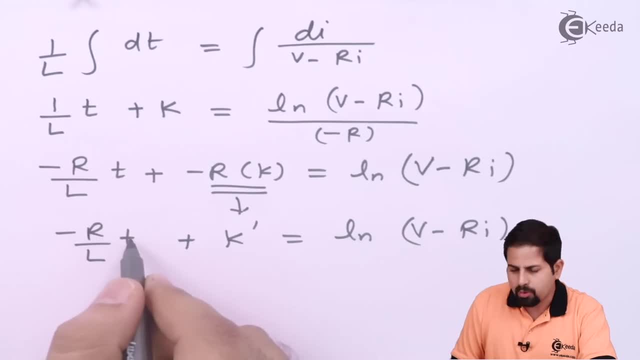 do here this term minus r by L into t by using rules of logarithms. I will write it as natural log to the base e and e raise to minus r by L into t, because if you solve this, this is the base e. if you solve this, you will get back the same term by using the rule of logarithms. 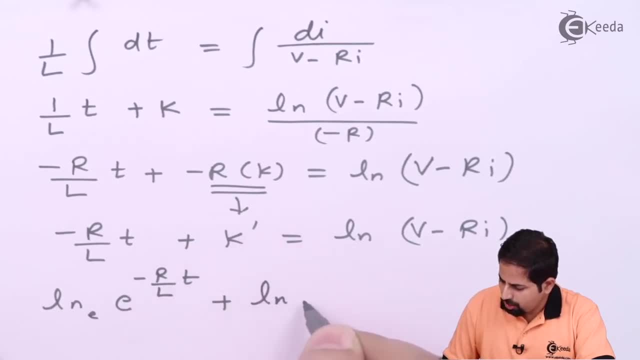 plus this k dash I will write as natural logarithm of some other constant. let us say it is small k. so that means this k dash is achieved by taking a natural logarithm of some another constant which is small k, which is perfectly fine. and then here you have natural log of V minus. 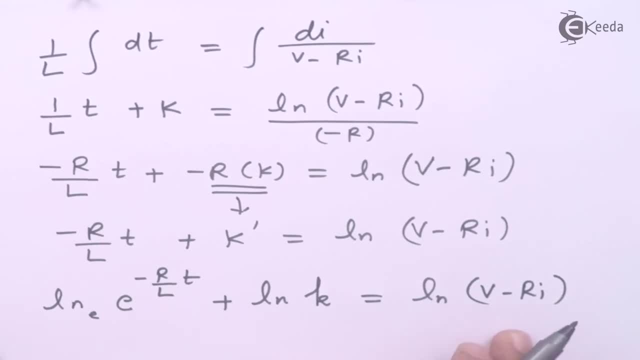 ri. Now here you have natural logarithms on both sides. see how we achieved it here. we just fitted in this natural logarithmic formula form Log e to the base. e will be means this term will come to this side, LHS side, and this will. 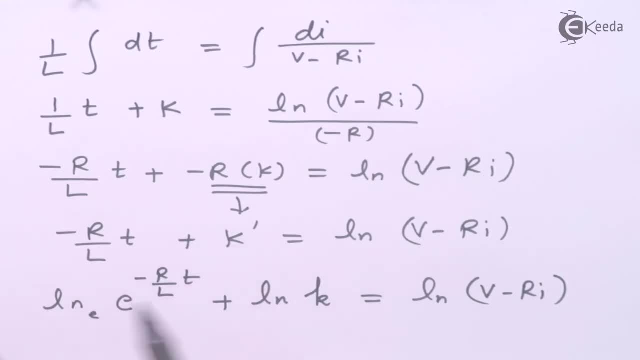 become 1 because natural log e to the base e is 1. then this k dash we have just written as natural logarithm of some other constant called as small k and here natural log of V minus ri, which is as it is Now. I can combine these two because there is plus sign I can. 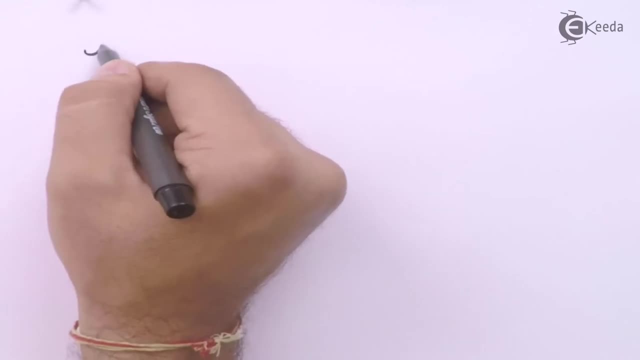 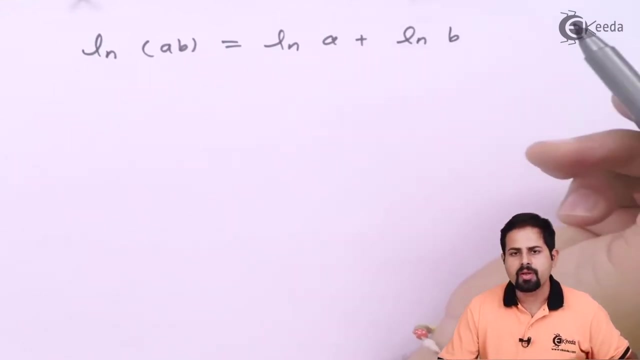 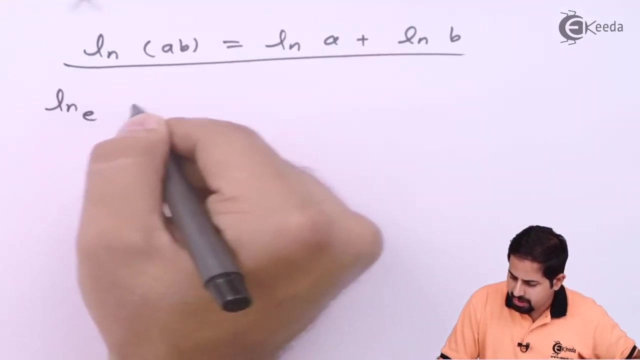 write this as multiplication of these two terms, because you know this formula, natural log of or any log of ab is equal to natural log of a plus natural log of b. So by using this formula, I will write: natural log to the base. e is equal to e. raise to minus. 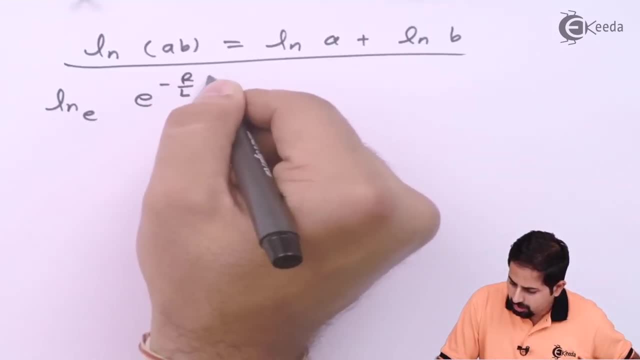 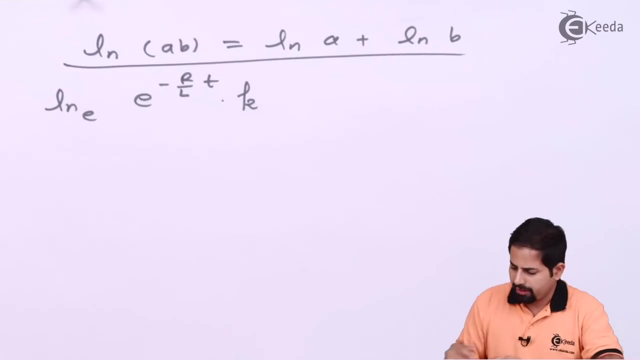 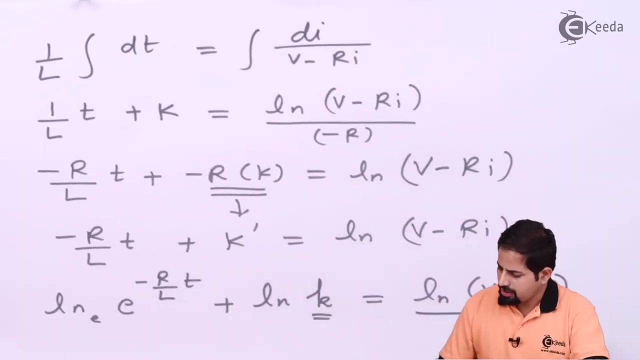 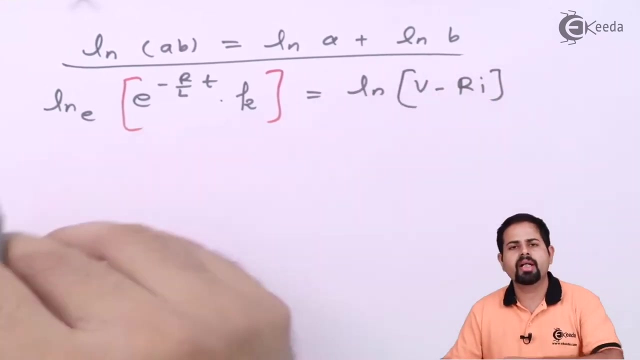 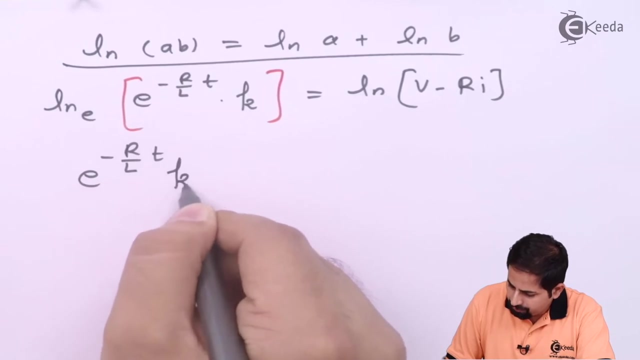 r by L into t multiplied by this k. so I will put it in bracket and that is equal to my RHS, which is natural log of V minus Ri. Now we can say that by taking antilog on both sides we will have e raise to minus R by L into T, into k is equal. 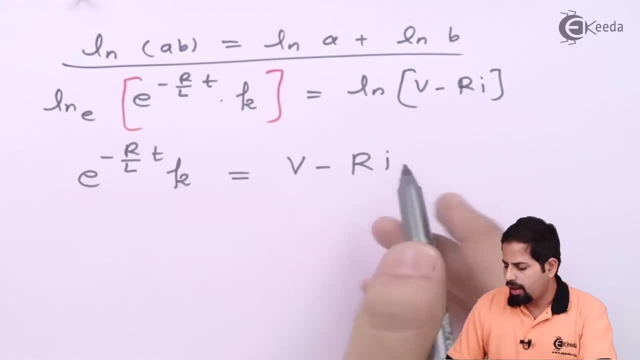 to V minus Ri. and now from this equation we can easily get: I, So for that I will take this Ri to left side, this term to right side. So Ri comes to left, which becomes positive, and this becomes V minus e, to the power minus R by L, into T multiplied by k. So we have 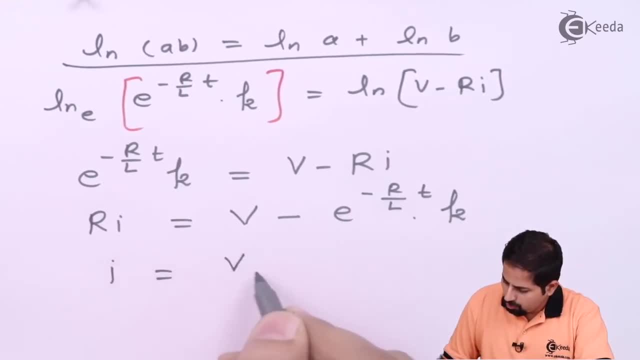 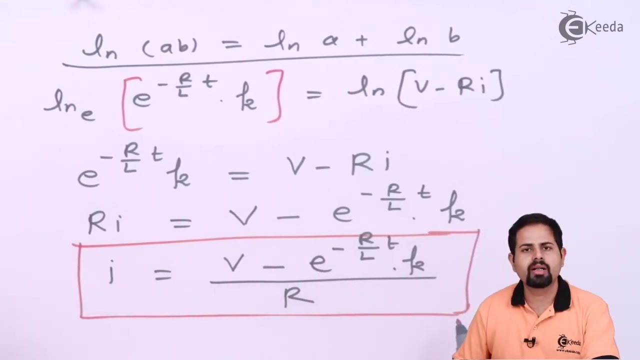 to get divided by R. So I will be equal to V minus e, to the power minus R, by L, into T, into k. the whole divided by R is nothing but the required. Now you will say, or you will wonder that what is this exactly we got? So we are yet. 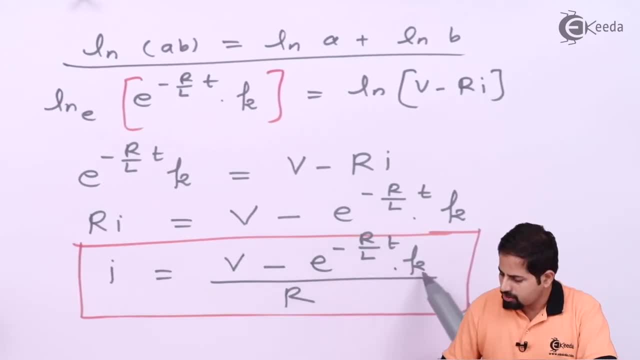 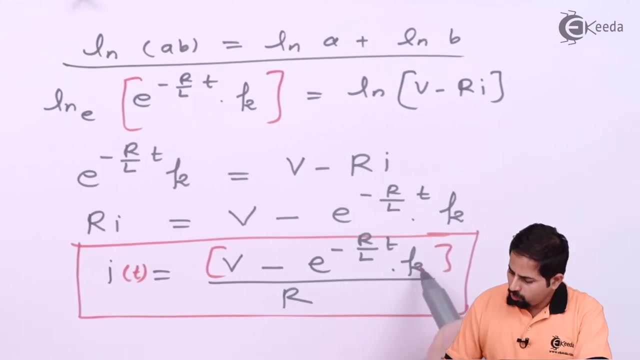 to put initial conditions by which we will get this constant k. So we got the value of I. I is obviously a function of time. everything is here means current and voltages are always functions of time. So I can write this: is I of t also. So now, if you want to get this, 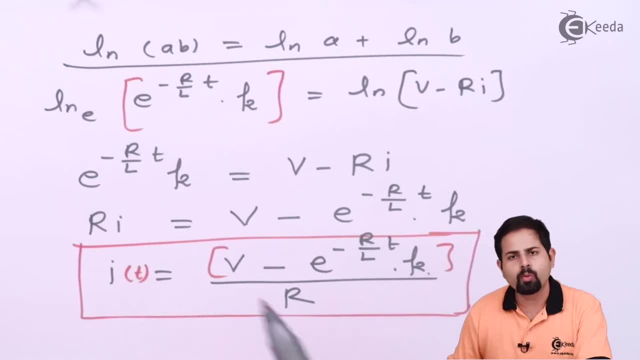 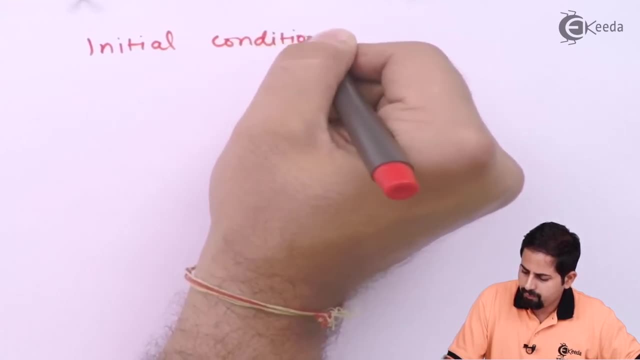 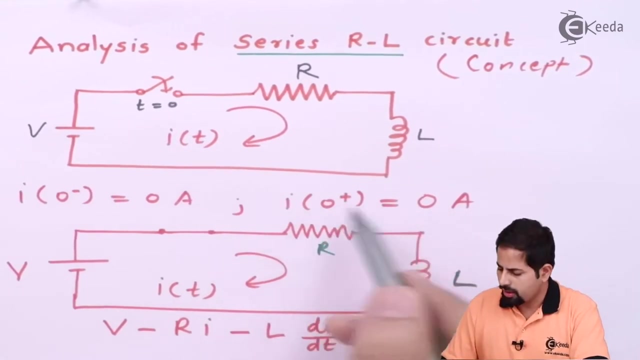 value of small k. that is a constant. you have to put initial conditions, And initial conditions tell us that which we have already written at 0 plus current is 0 ampere. So at time t equal to 0. also current is 0.. So initial conditions are at: 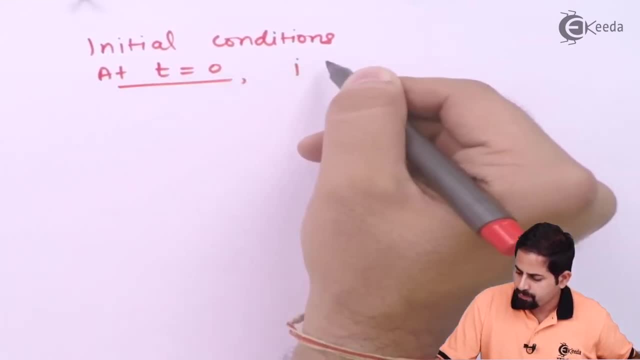 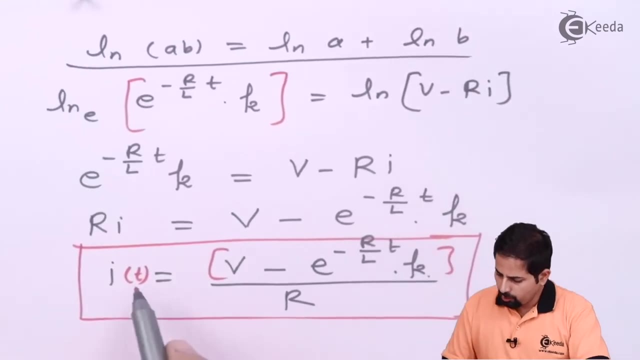 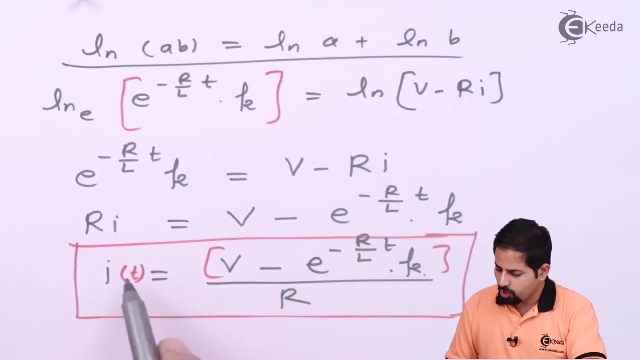 t equal to 0, I of 0 is going to be 0 amperes, And so when you put t equal to 0, you will put t equal to 0 here also, and it is easy to solve. So I of 0 is going to be 0. So write this as equation number. 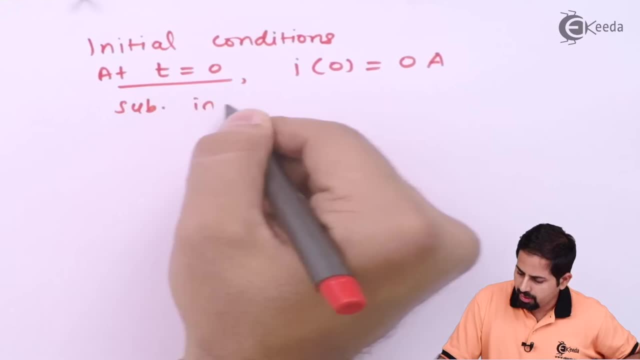 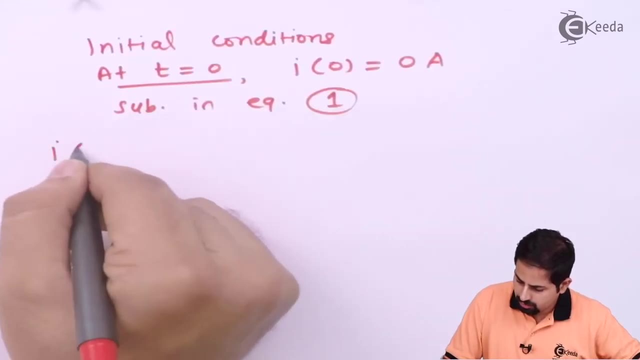 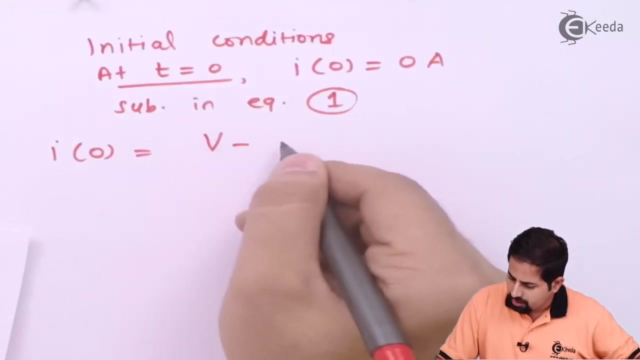 1, substituting in equation 1 this part I of 0 is equal to- because we have to do it at time- t equal to 0, V minus e to the power. now this t is 0. 0 into anything will be 0. So 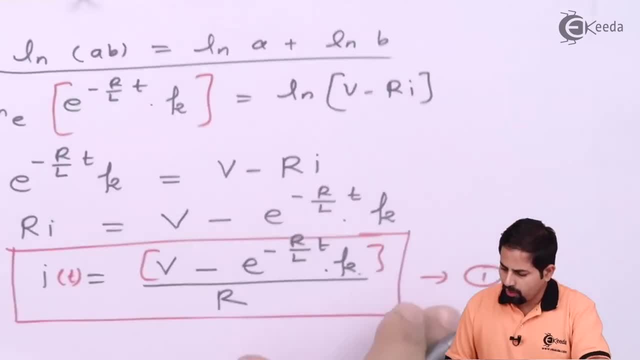 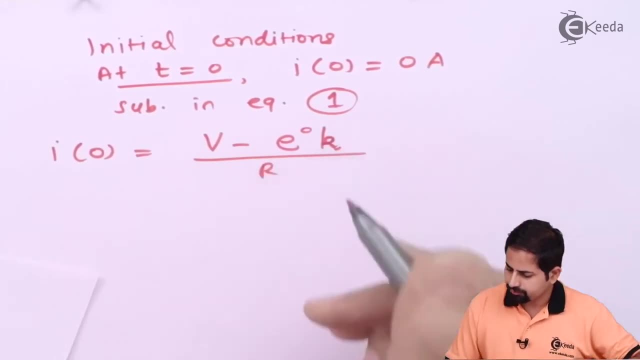 e to the power 0, which is going to be 1, into k by R. this is k And so current is 0, so I will write this 0 here, V minus k by R, and this R also goes here. it becomes 0. So for: 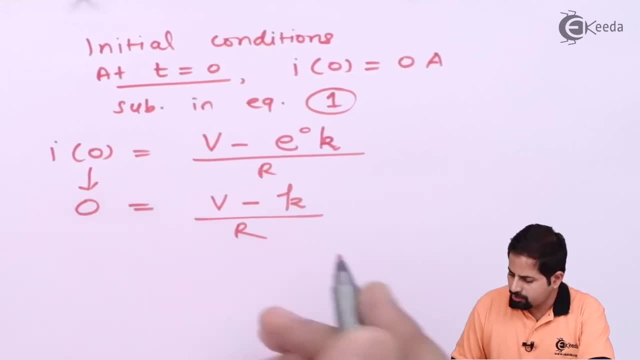 becomes 0, or this R multiplied by this LHS will become 0 and this K will be equal to V. So finally, we have got this constant K. Now let us say that this is equation number 2 and substitute equation 2 in equation 1.. Now, what is equation 1?? By the way, this: 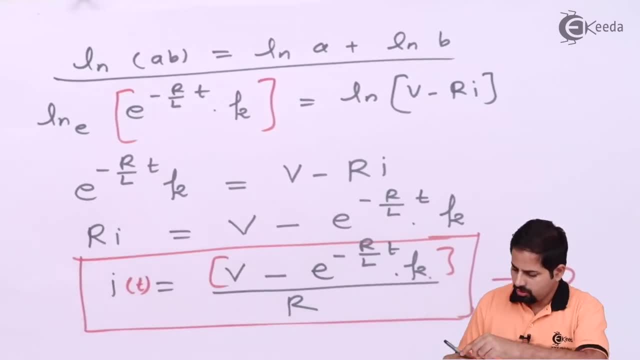 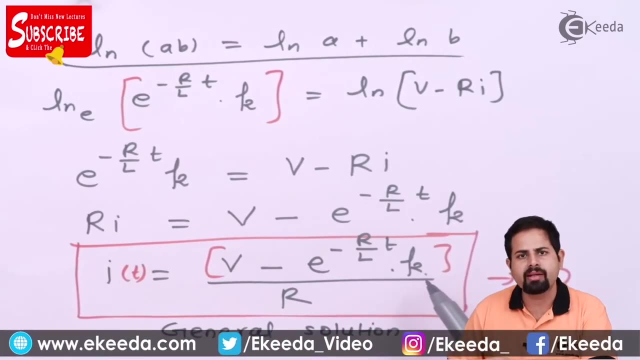 equation 1, which we have got, is called as general solution because it is applicable generally. When you calculate the value of constant K by putting the exact values of current and voltages, it becomes a particular solution In maths. we have done this when. 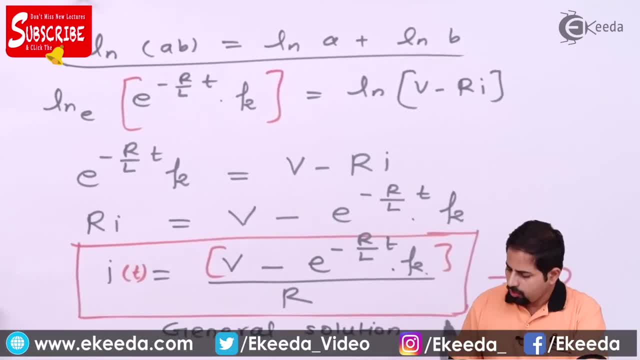 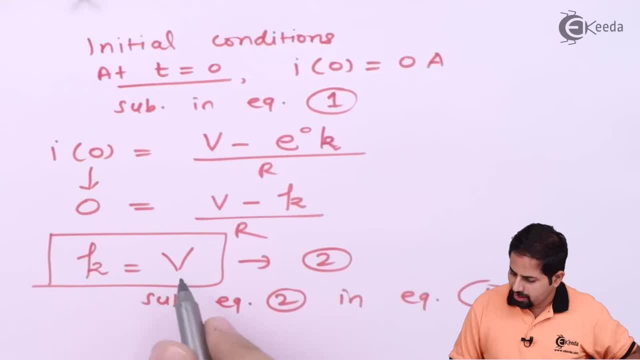 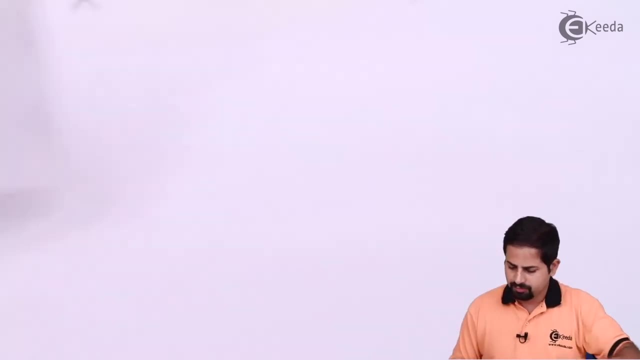 we solved homogeneous equations. So now, if you want to get the particular solution, we will have to substitute this value of K, and so we got K equal to V. So instead of this K, I will put V. So I will get I of t, which I will do in the next page. 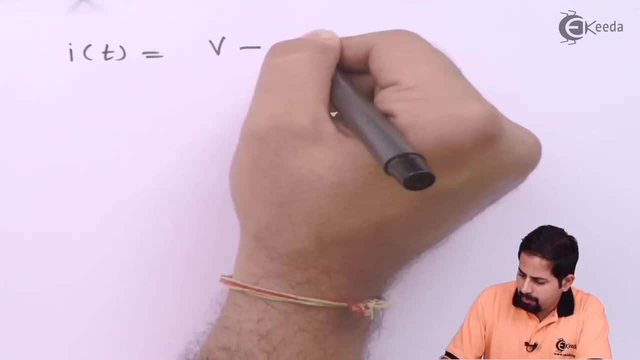 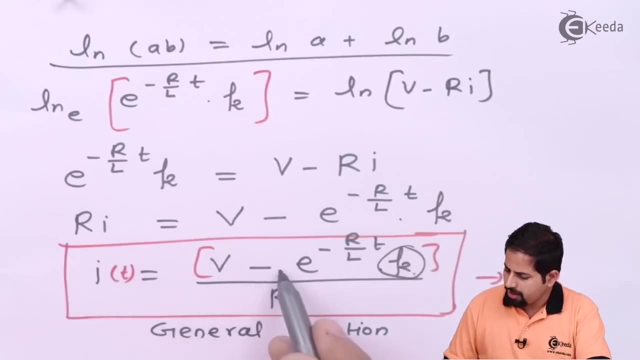 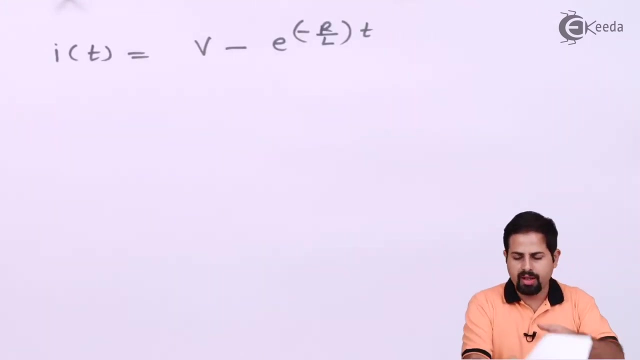 So I of t now is V minus e raise to minus R by L into t. I of t: V minus e raise to minus R by L into t, multiplied by this small k divided by R. So multiplied by this small k is nothing. 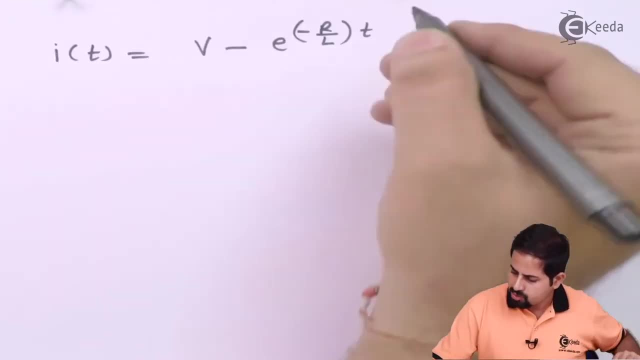 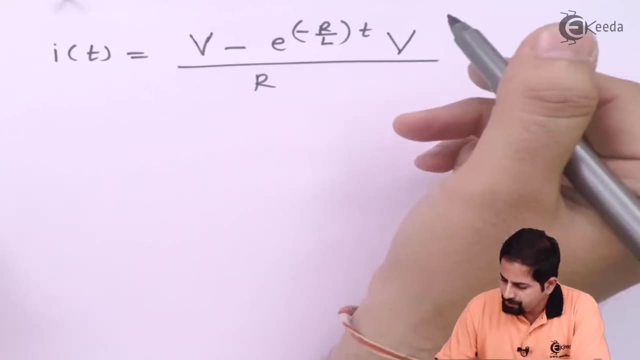 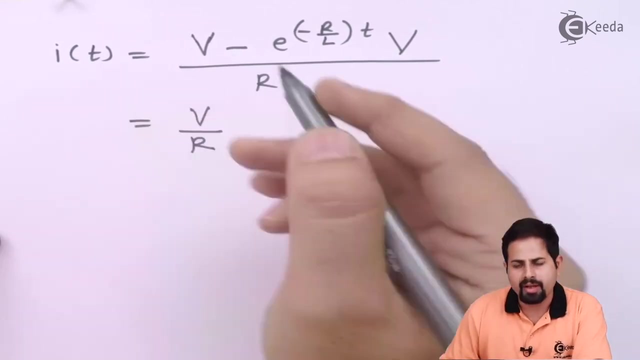 but that we have obtained K equal to V, capital V. So it is multiplied by capital V divided by R, This is same. capital V means voltage. So now we have obtained K equal to V. So now I can take this V by R, or we can, we will take it common later, V by R minus V. 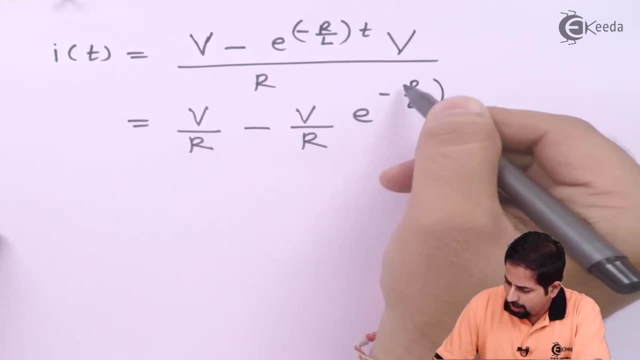 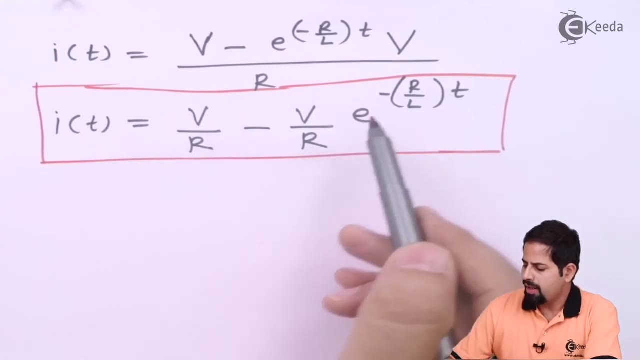 by R e to the power minus R by L into t. This is nothing but I of t which we have got. So we got V by R minus V by R into e. raise to minus R by L into t. This is the final. 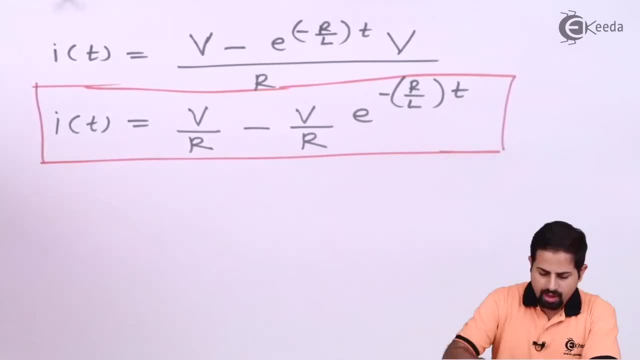 form of current for the given case of series R L circuit. Now again, what we can do is we can take this V by R, common, and then we can write it as 1 minus e to the power minus R by L into t. This is also one way to write which is good for drawing the exact waveform. 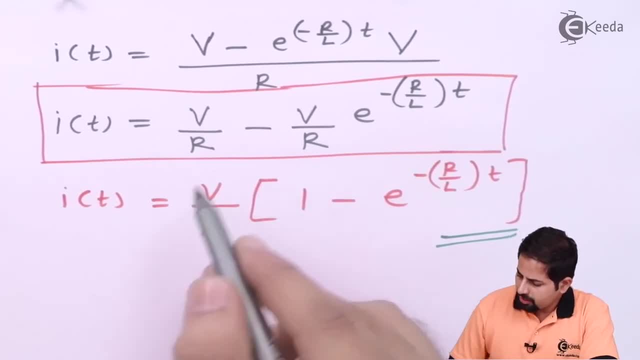 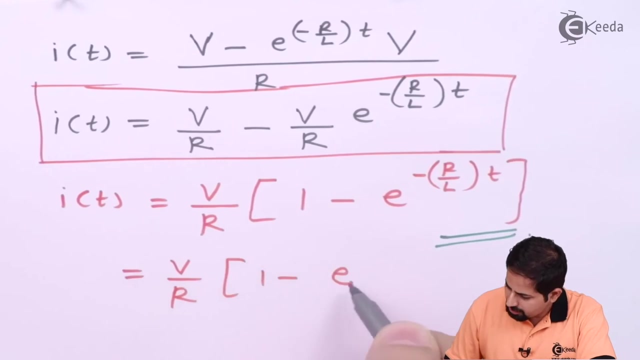 or So that means the current is nothing. but it depends on, obviously it depends on time And there is a constant here, R by L. So there is a way to write it So: V by R in bracket 1 minus e raise to minus t divide by this R by L. if I put it in denominator below this: 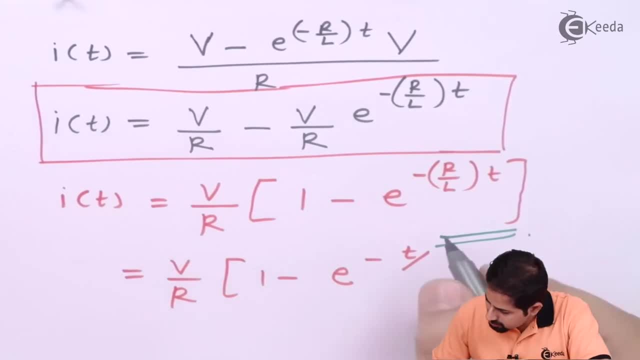 t, it will be L by R, So that I will write like this: L by R. See, I will repeat again: this is minus sign as it is here, this t also as it is. instead of R by L, I am taking this R in below this L in denominator, So it becomes L by R. the use of this is: we can now generalize. 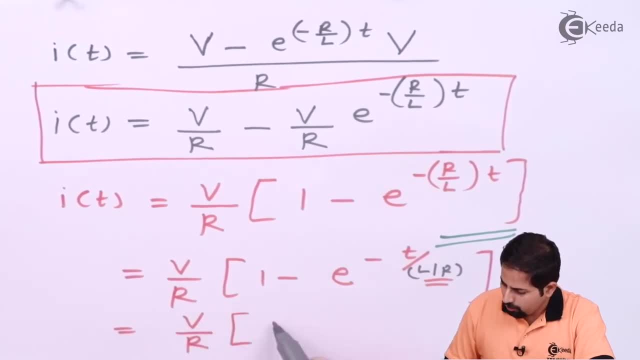 it. it is V by R into bracket e, raise to minus e to the power minus t. divide by tau, where this tau is called as time constant. because we have taken series RL circuit, this tau, which is L by R, So L by R will be the time constant of series RL circuit. So I will write it separately. 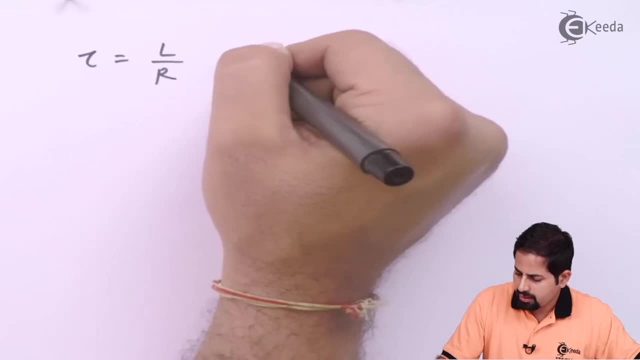 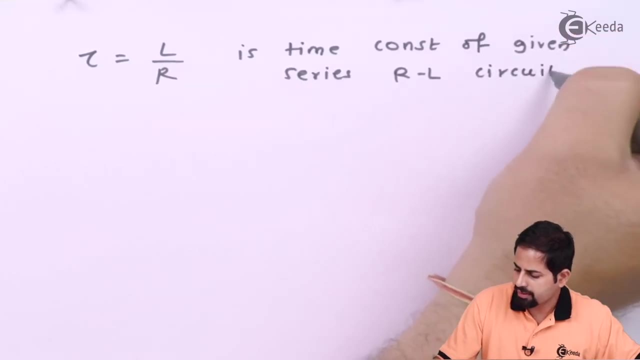 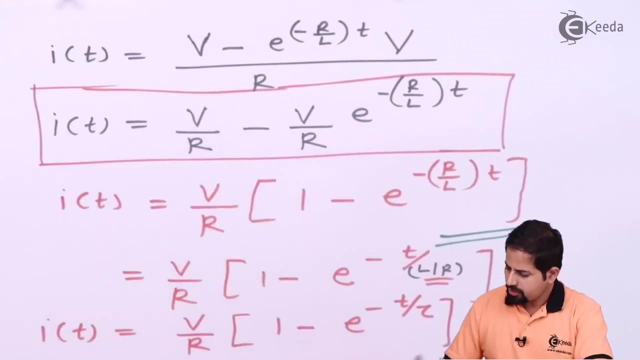 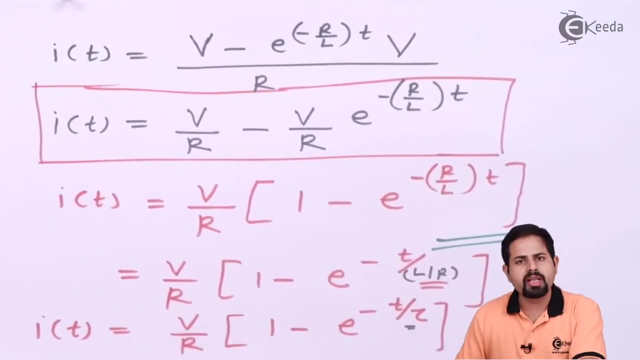 now tau equal to L by R is time constant of series RL circuit. Now how to plot this waveform. So it is my e to the power minus t by tau. So how to plot it, So we will plot it for. 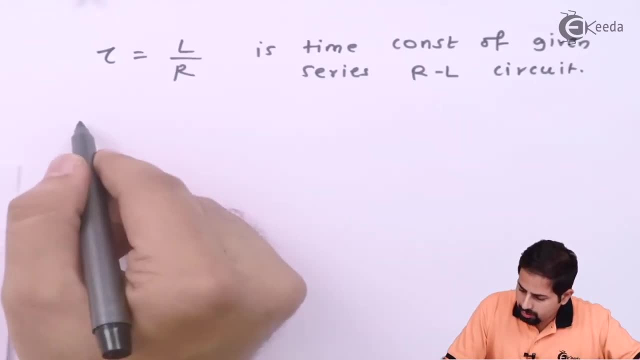 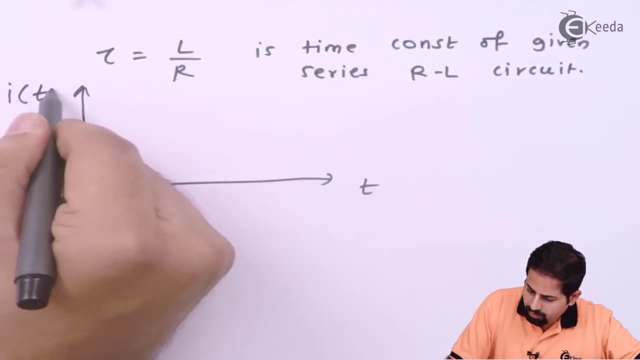 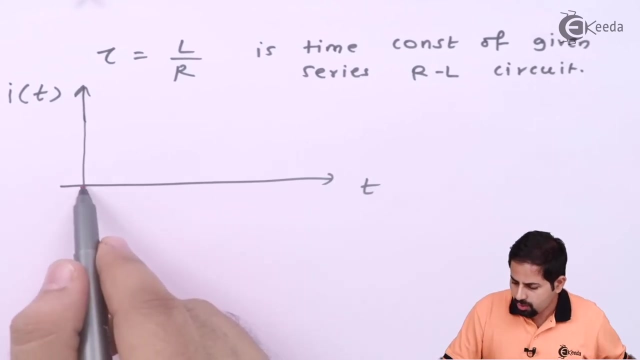 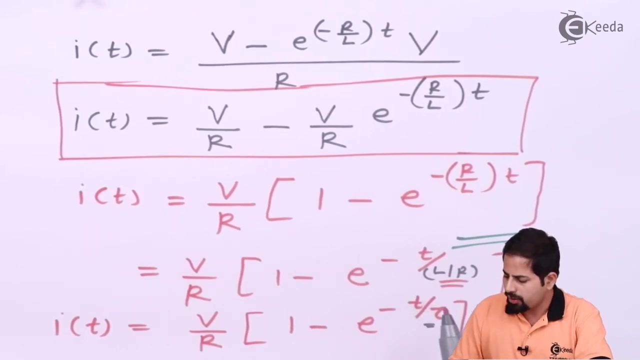 t greater than or equal to 0.. So, to plot it like this, this is going to be t, this is going to be I of t. and see our graph. starts with time t equal to 0. this point, and when time t is 0, if you substitute it here, e to the power, 0, which is going to be 1 and 1 minus. 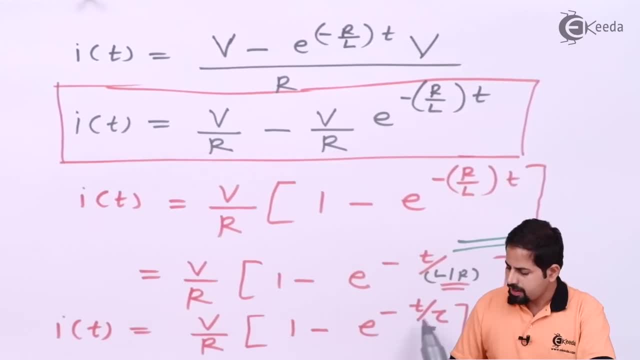 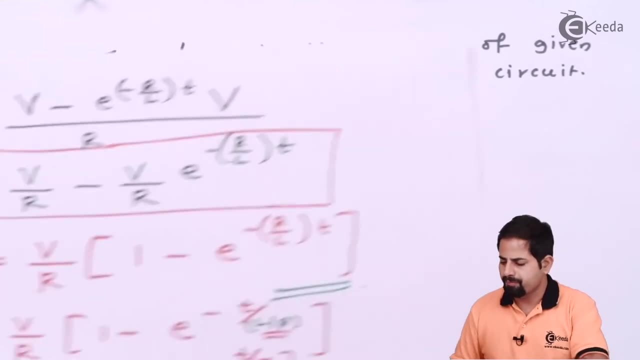 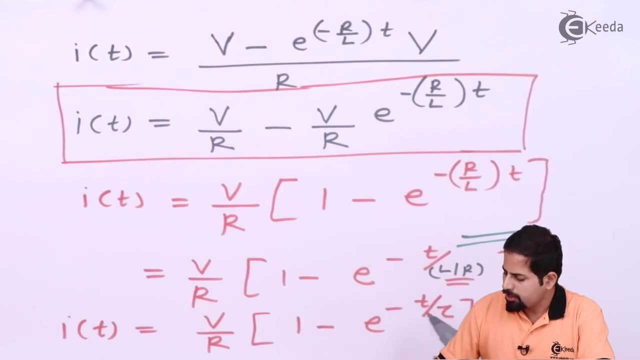 1.. So this factor will become 1.. So time t is 0, this e to the power. 0 will be 1, 1 minus 1 will be 0 and our current will be 0. So this will be our starting point for current. well, when this t takes the value of tau, this: 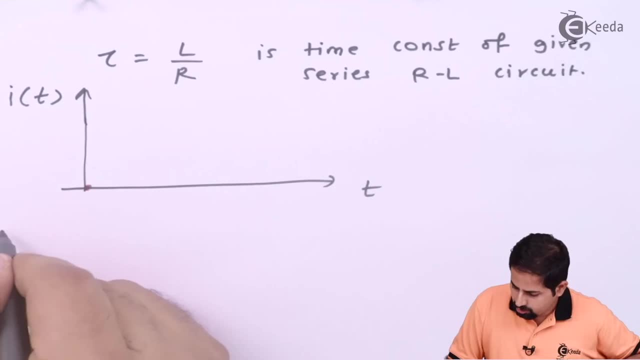 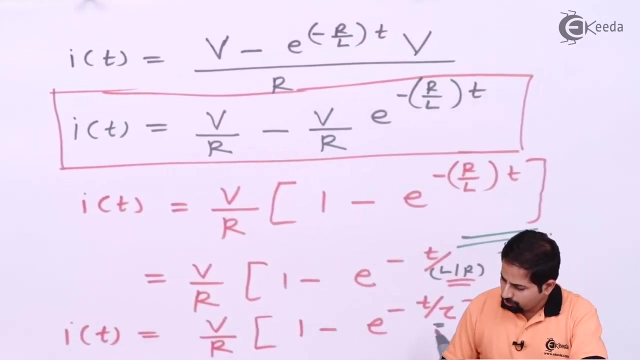 will become e to the power minus 1.. So we will write it at t equal to 0, first case. at t equal to 0, you get I of t equal to 0. Then at t equal to tau, I will get I of tau equal to I of tau equal to V by R 1 minus when. 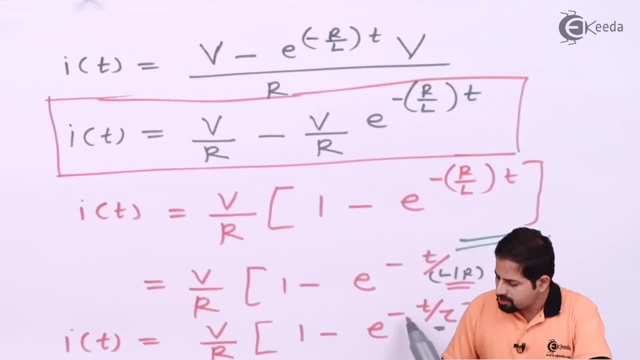 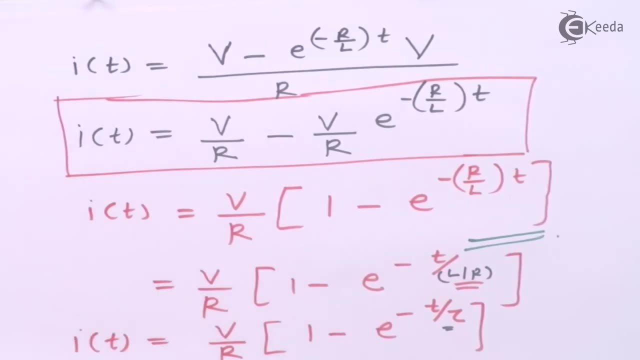 t and tau. both are same. it is going to be e to the power minus 1.. So d into d of time minus 1, you can calculate 0.3678.. So 1 minus point, this factor comes out to be 0.3678.. 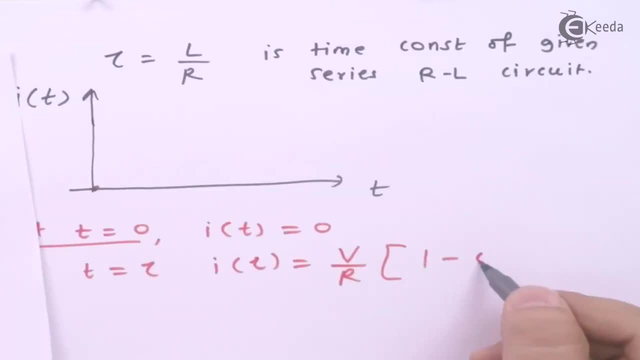 Yes, What is my? k additions 1 is lost. and now, if you do that, the calculation, So this is going to be V by r into minus 0.632.. So initially it is 0,, the current value is 0,, when time increases then it becomes 63%. 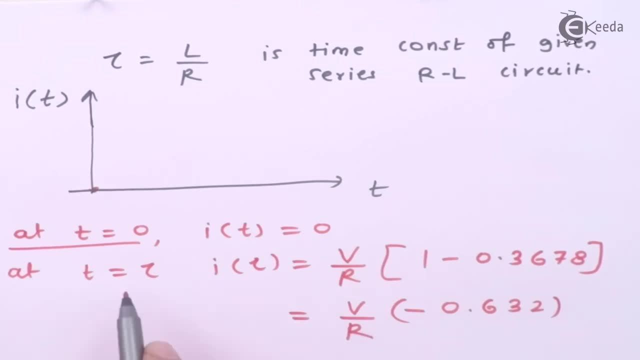 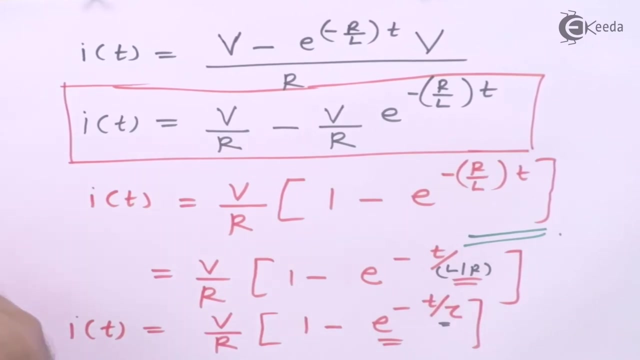 of V by r. Similarly, if you keep on doing this, when you go to t equal to 5 tau, you will almost go to 98% of the value of V by r. and it is but obvious that when you substitute this t As infinity, because we are doing the analysis for t greater than 0. 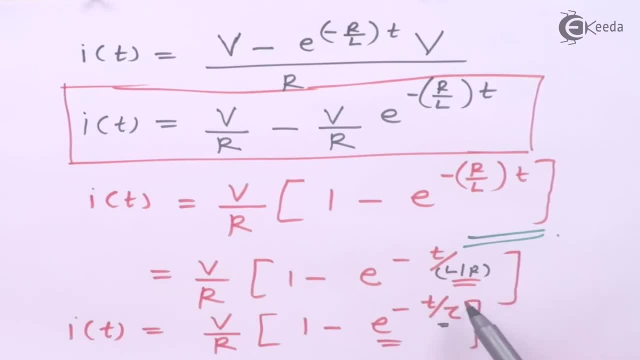 So when this t increases or it becomes very, very large, suppose t becomes infinity- e raise to minus infinity, which is 0. So at t equal to infinity or larger values of t, this factor will become 0 and your answer will become solely V by r. 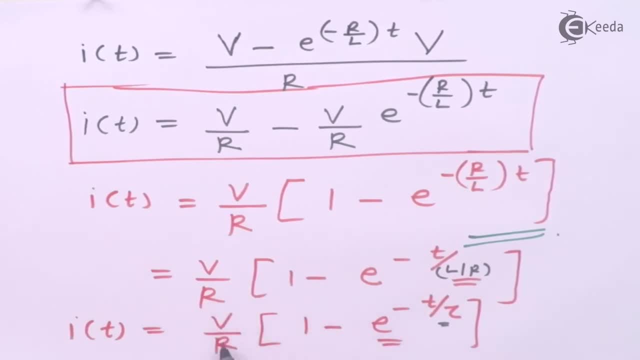 So the final value for current will be. maximum value will be just V by r, because 1 minus 0 will be 1.. And why this will be 0? Because t is going to increase. why it is going to increase? because we have plotted it on. 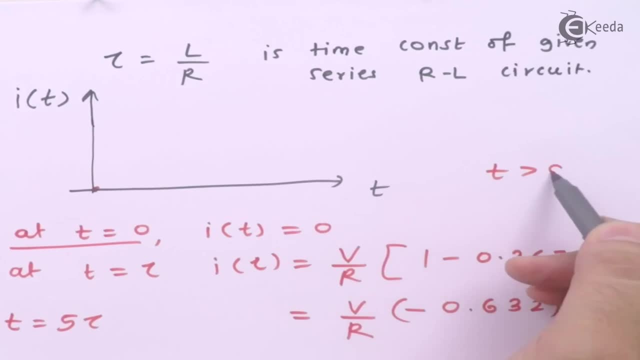 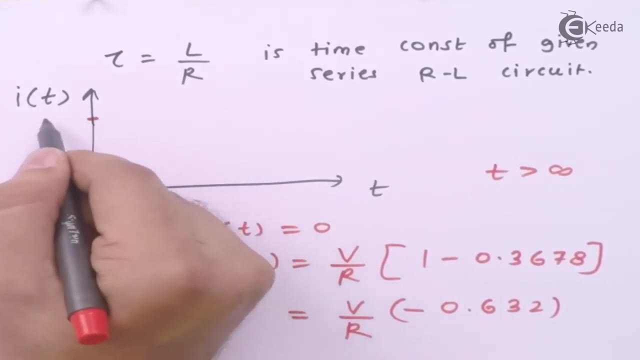 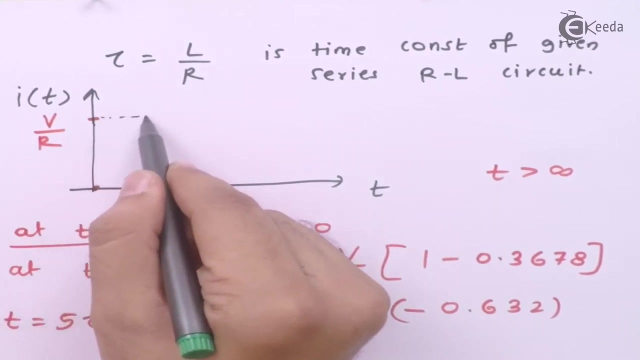 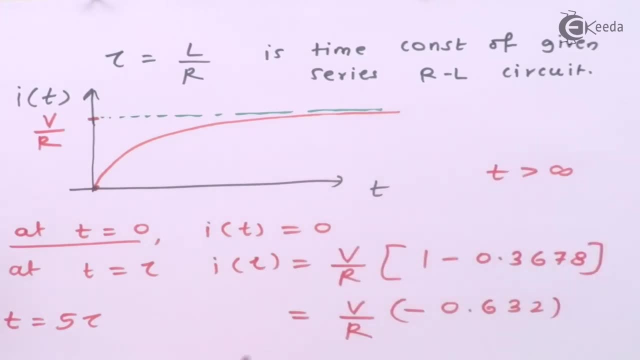 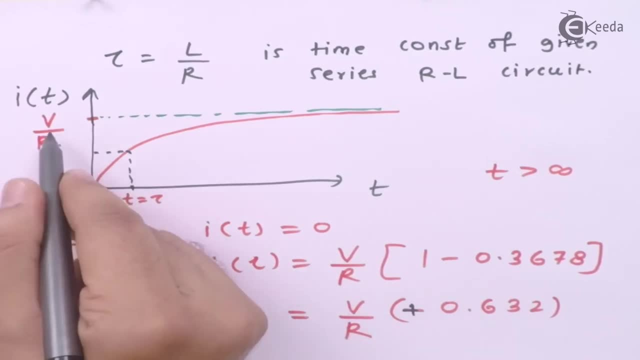 So 63 percent. so 63 percent of V by r. so we can write this as 0.62 of V by r, and so on. you can do it for 2 tau, 3 tau, 5 tau. once you are done with 5 tau, your corresponding value will. 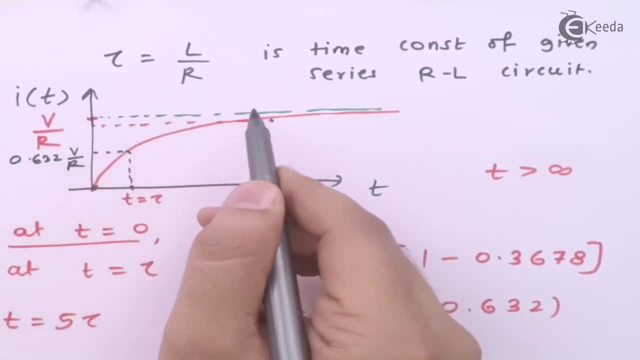 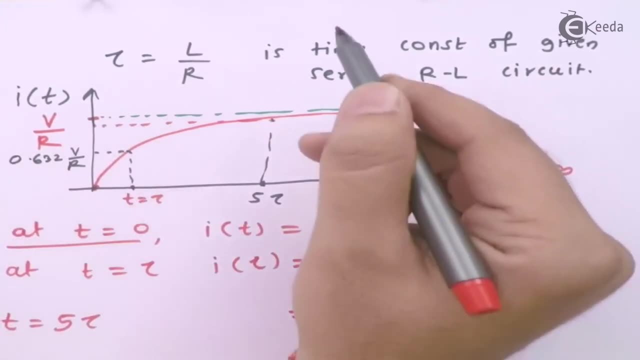 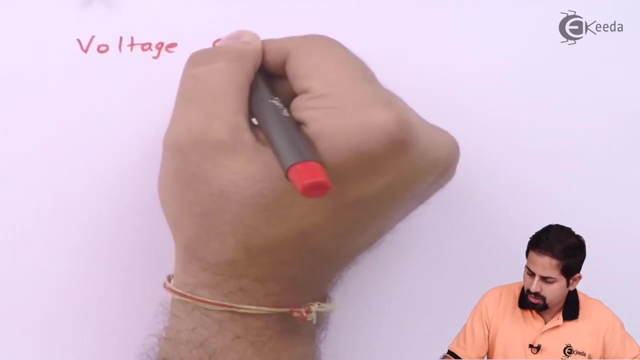 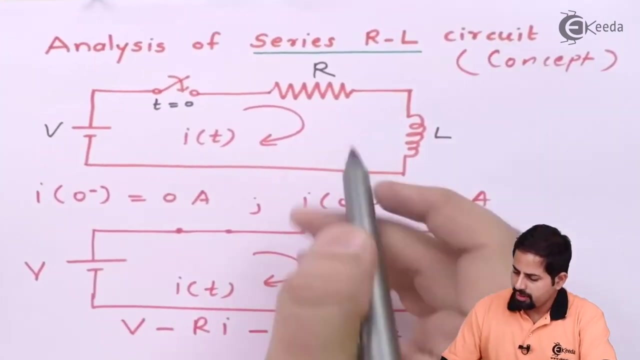 be almost 98 percent and when you go on increasing this it will be almost equal to v by r. so this is the graph of current. now what is the voltage across? resistance and inductor? that also can be calculated voltage across, because our circuit is like this: if you refer to this circuit, r and 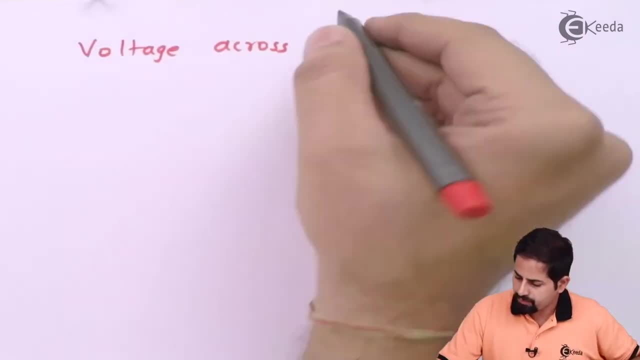 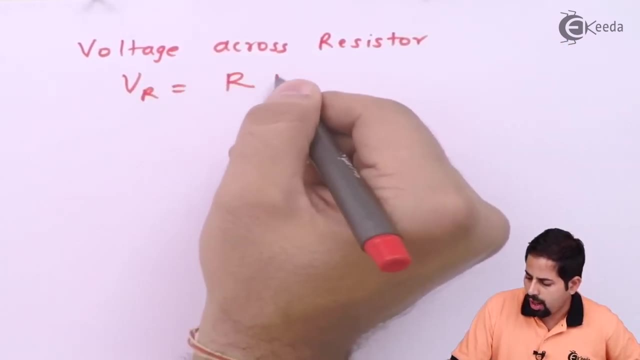 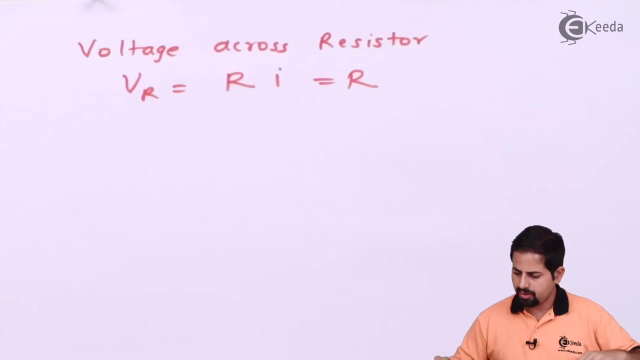 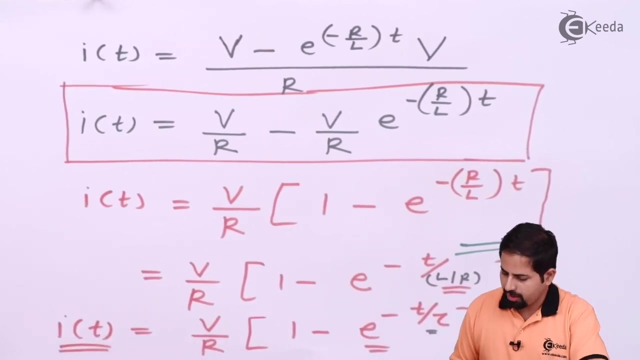 l. so first we will calculate voltage across resistor. so v across r is nothing but equal to r into i, and we have just got what is i. i is nothing but v by r into 1 minus e, to the power minus t by tau. so i will substitute this value of current here. 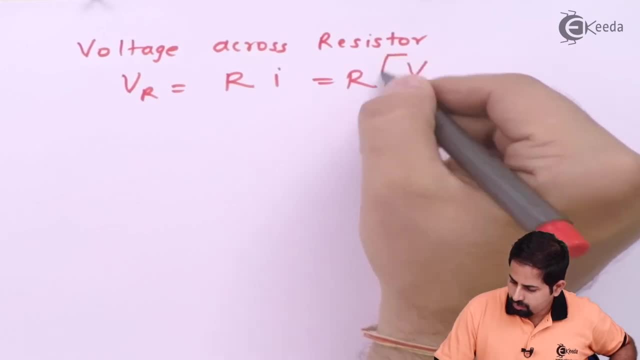 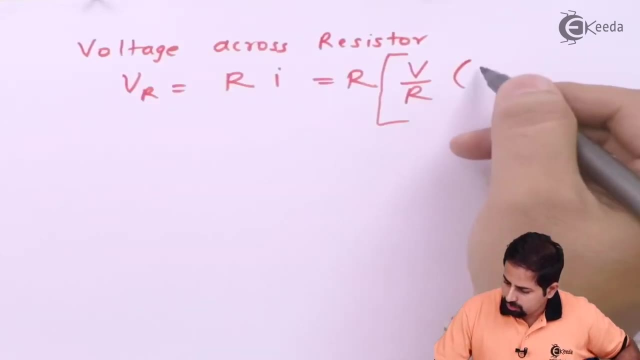 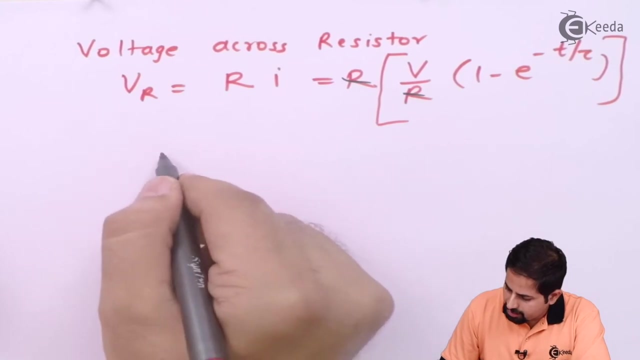 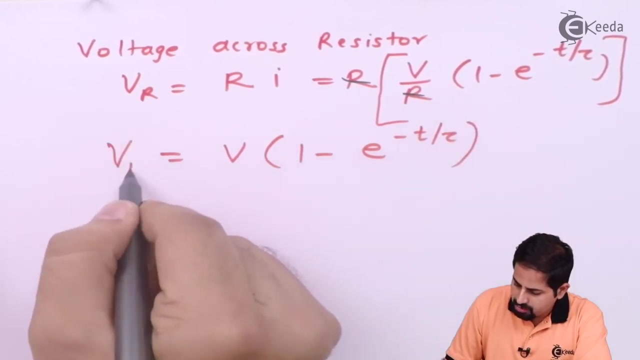 so r into v by r into 1 minus e to the power minus t by tau. tau is time constant equal to l by r. so this r and r will get cancelled and what we will get is nothing but V into 1 minus e to the power minus T by tau. this is voltage across resistors. 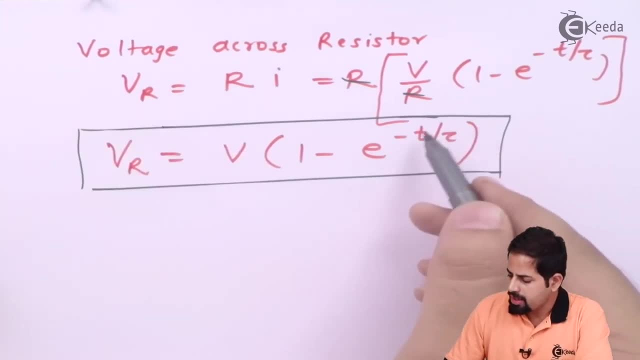 How to plot it Approximately how to plot it. So when time T is 0, e raise to 0 will be 1 and 1 minus 1 will be again 0. So again at start, voltage across resistor will be 0. 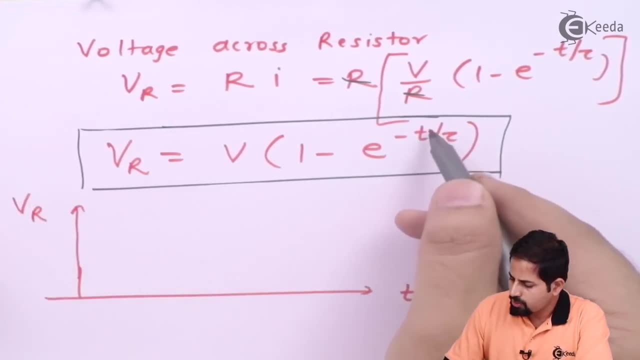 See again: I put time T equal to 0, e to the power, 0 is 1, 1 minus 1 is 0. So it is going to be 0 again. and when I put T equal to infinity again, e raise to minus infinity, it will become: 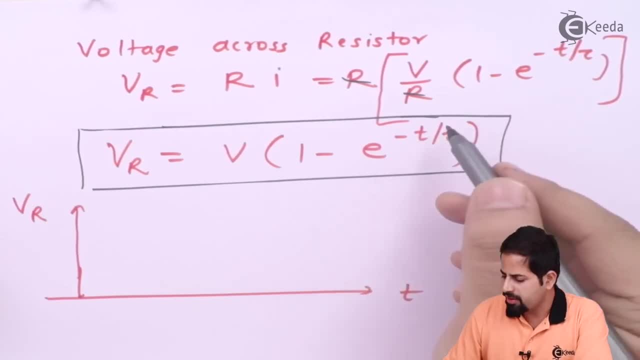 when I substitute at T equal to infinity, e to the power, minus infinity, will be 0,. 1 minus 0 will be 1.. So it is going to be V, So maximum value for it is going to be only V, and the graph will be, and so on. 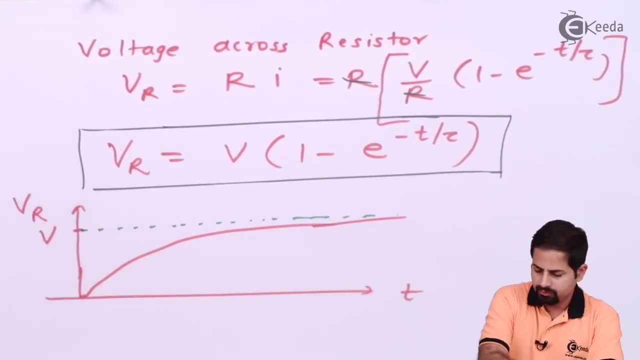 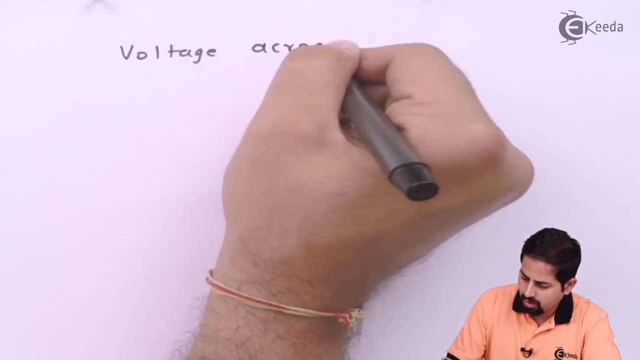 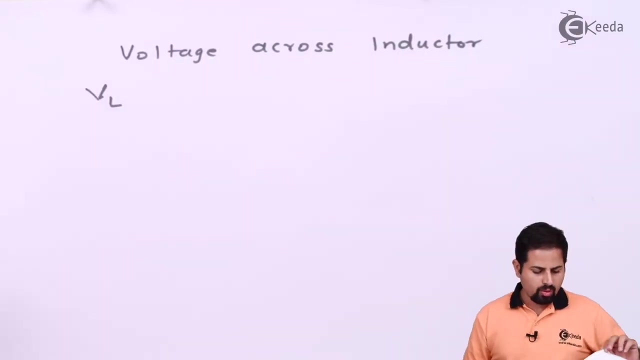 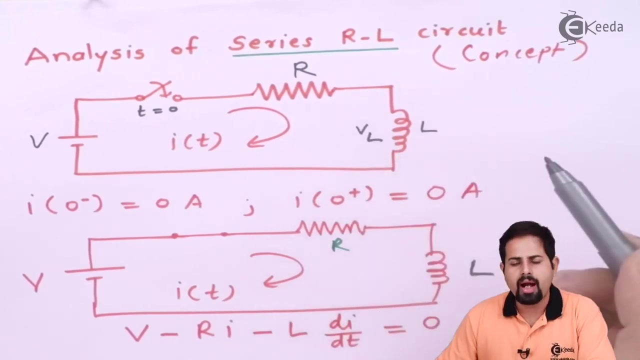 Now what will be the voltage across inductor? So for that you will write voltage across inductor, that is VL, and if you see the original diagram, there is an inductor. So the voltage across inductor is nothing but VL, and that VL has a formula. this is equal to L into. 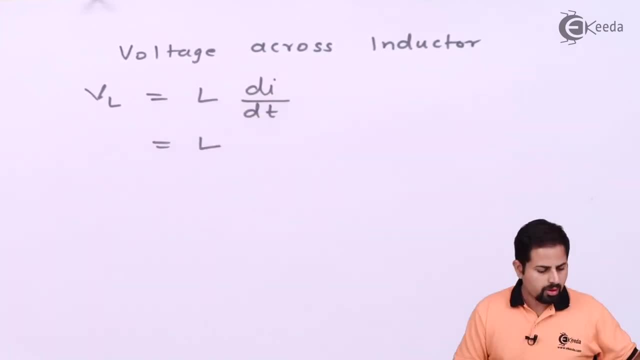 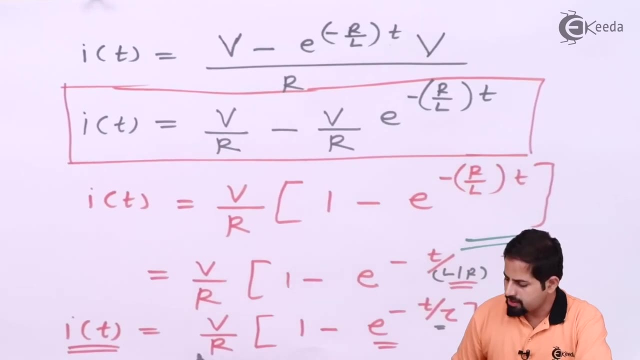 dI by dT, So it is going to be L into, or the value for a current I which we have obtained and we will use it. It is this value, V by R, 1 minus e to the power, minus T by tau, So it: 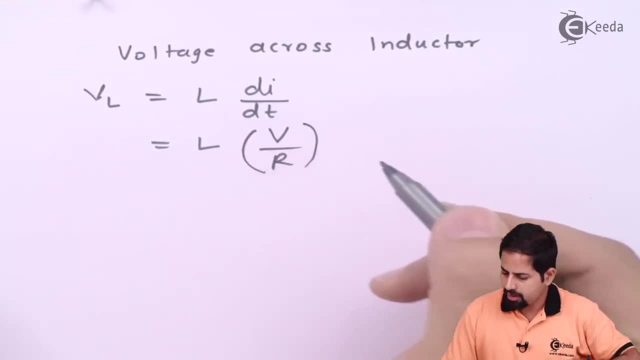 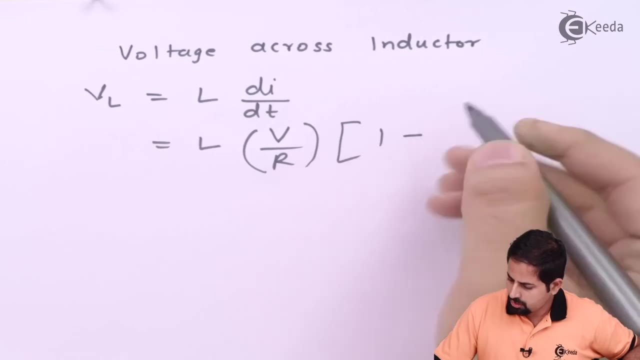 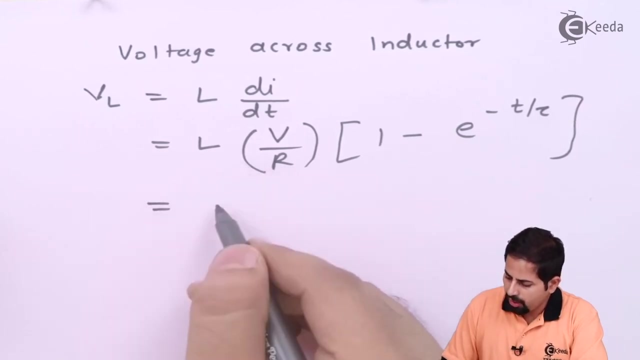 is V by R 1 minus e to the power minus T by tau. So now, if you solve it, you will get L into V by R 1, it is going to be L into V by R, or we have take the derivative of this. So here I will write Follow. 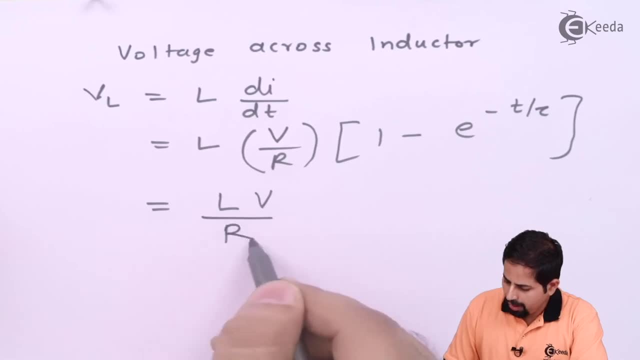 the draw method on the DT graphical is equal to L, D by B by DT. I will write D by DT of this, So derivative of this term is required. So instead of this we will get: B by R will be a constant, it will be outside. This is nothing but this y optimal ance value. I am writing like this: el n integral of this Product x by Tribe x valim protecting itself will be. So instead of this, you will get the value of the right side plus the 몸 over this нож. So derivative of the right side, desseقطants and擊 bias in the. 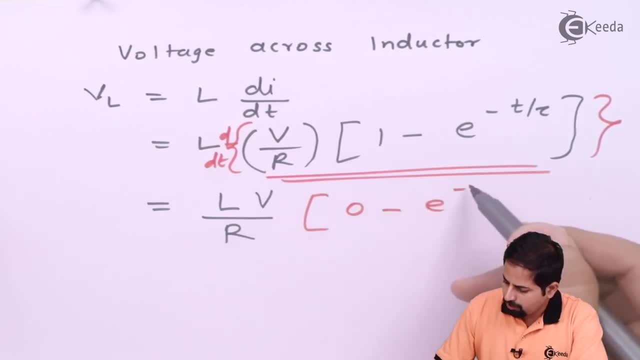 this term will be again 0, minus e to the power, minus t by tau and coefficient of it. that will be multiplied and that will be minus 1 upon tau. so this first term is going to be 0 because it is a constant, and so it is l v by r. this minus will come minus and minus will become plus, and so it. 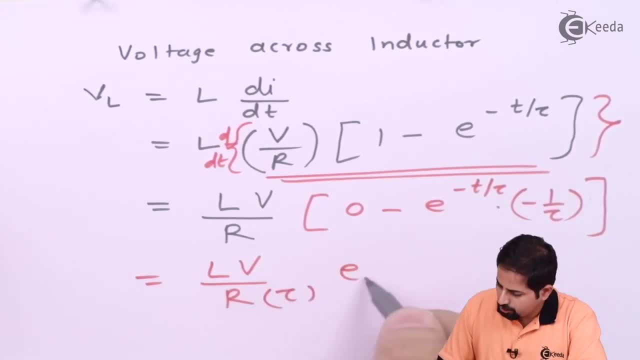 will become if tau will come here and e to the power minus t by tau, and we know the value of tau. tau is nothing but l by r, so this is going to be equal to this l. i am writing as it is. this r also i am writing as it is now. tau is nothing but l by r, so l divided by r. 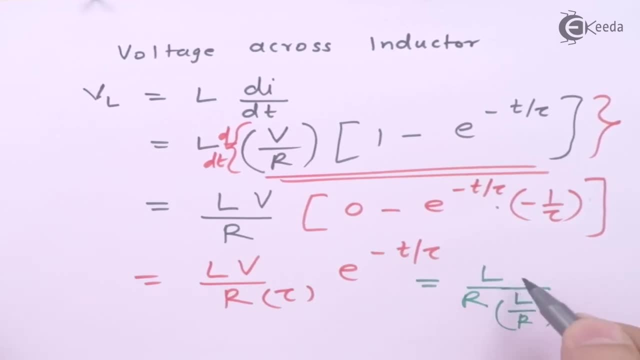 so there will be some cancellation and here v will be as it is, this v. i am writing e to the power minus t by tau, and when you solve it you will get here that this l and l will get cancelled. this r and r also will get cancelled. 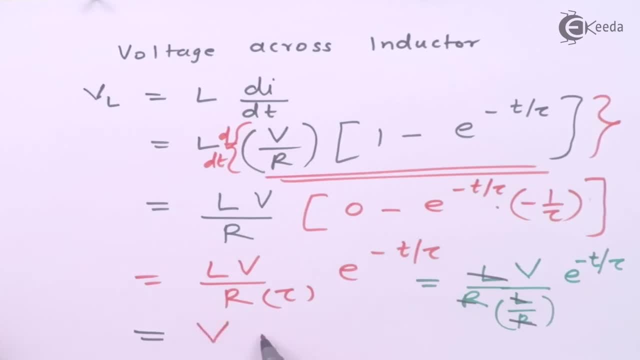 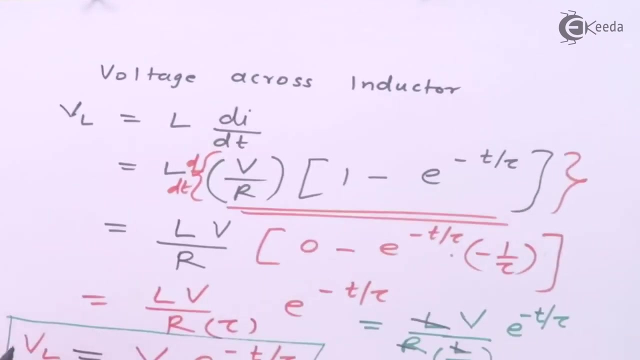 and so what you will get is nothing but v into e, to the power minus t by tau. this is nothing but voltage across inductor. so i will put it in bracket and we will draw the graph in the same graph which we have drawn for resistor. so here you can see: the voltage across inductor is capital v. 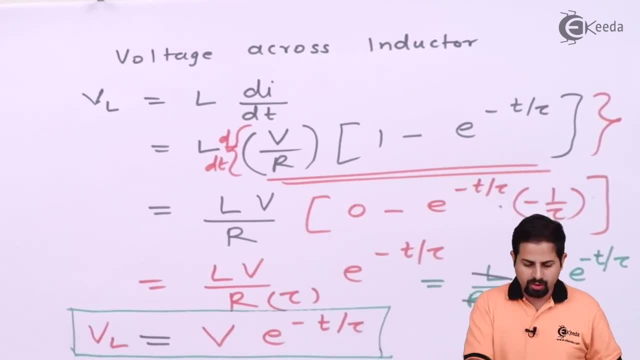 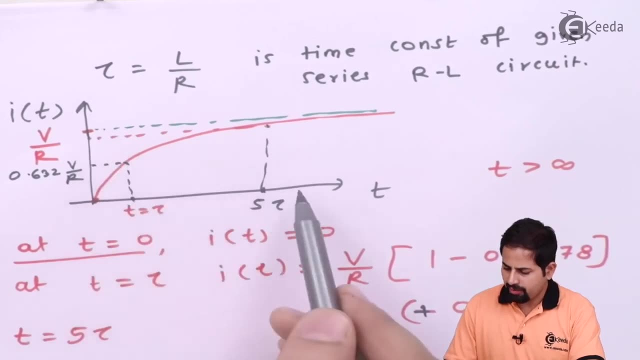 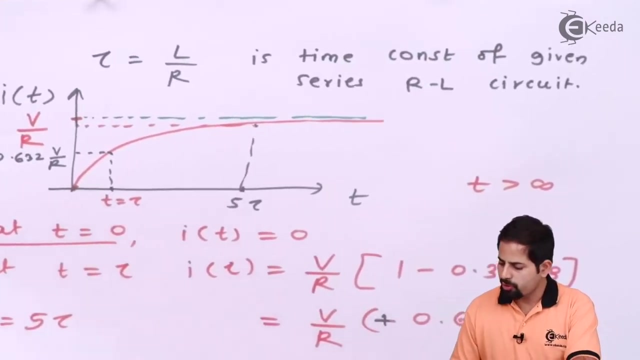 into e raise to minus t by tau. so if you see the graph for resistor, we will. we can draw in the same graph or we can draw different also. so if you want to draw in the same, well, put t equal to 0, because first time t is 0. so when you put t equal to 0, e raise to 0 will be 1. 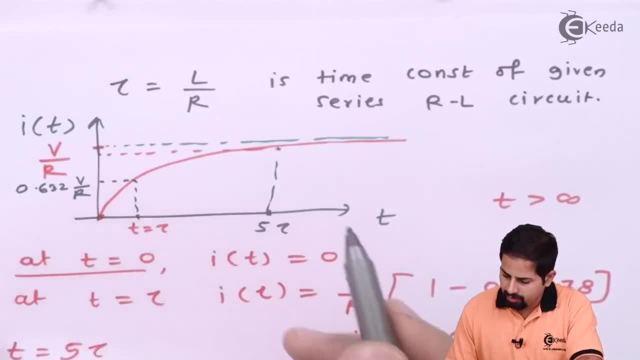 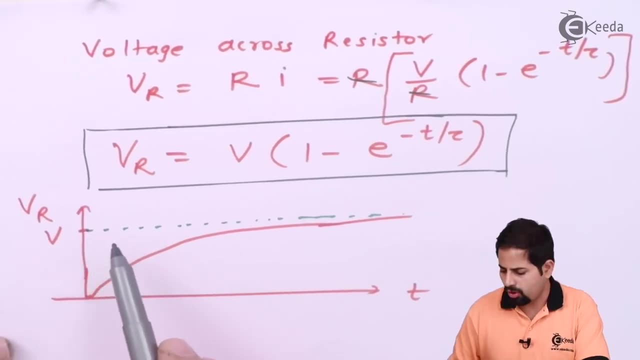 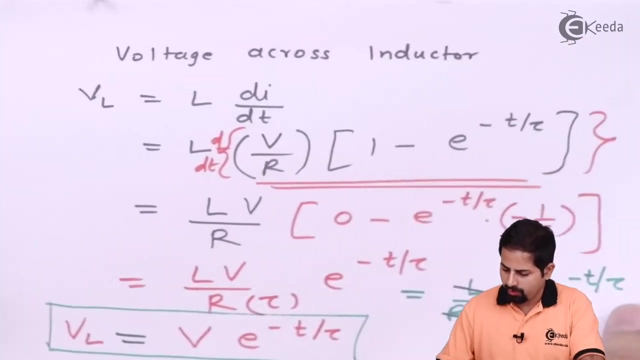 and your value will be capital b. so you will start. no, this is not the graph. so here we will draw the graph in the same graph where we draw the voltage across resistor. we draw this graph is for voltage across resistor. now you see the formula. voltage across inductor is v into e. raise to minus t by tau. 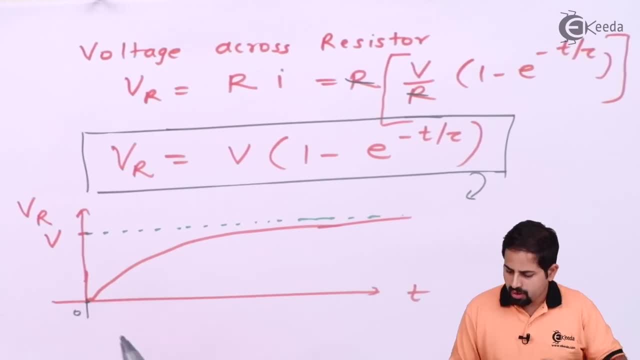 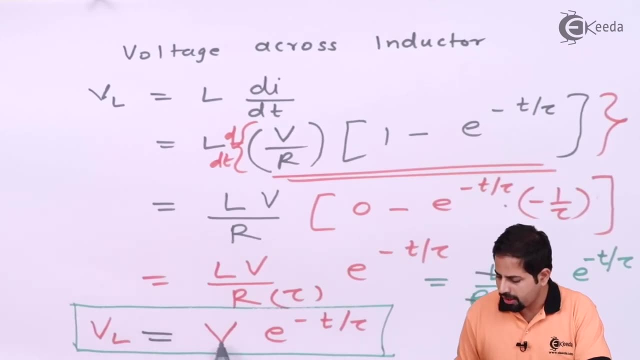 our first time instant it t equal to 0. so when you put t equal to 0, e raise to 0 will become 1 and at t equal to 0, you will get v, l equal to only v. so you will start from here and see as this: 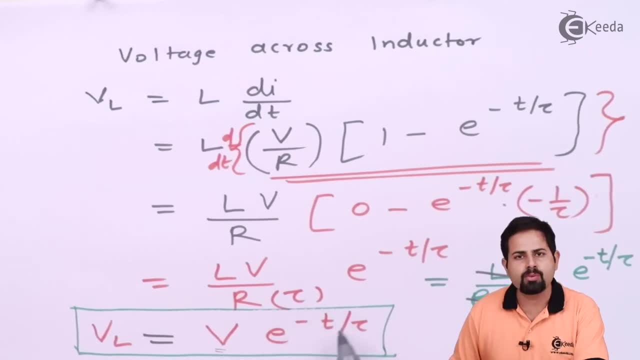 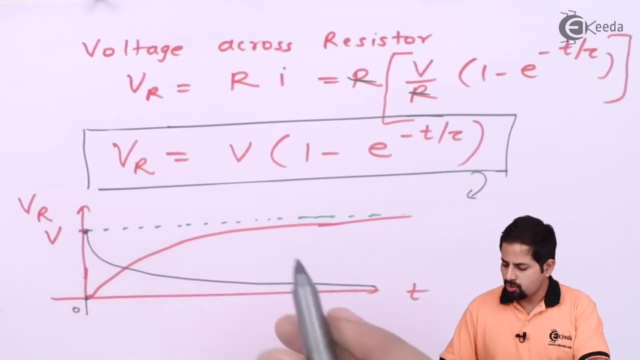 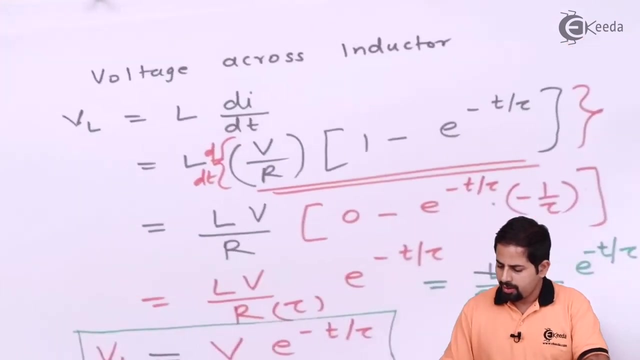 t keeps on increasing because it is an decaying exponential, the graph will be decaying like this and so on. so this is graph for L and this is graph for VR. as T becomes 1 tau, 2 tau, 3 tau, 4 tau and 5 tau as it. 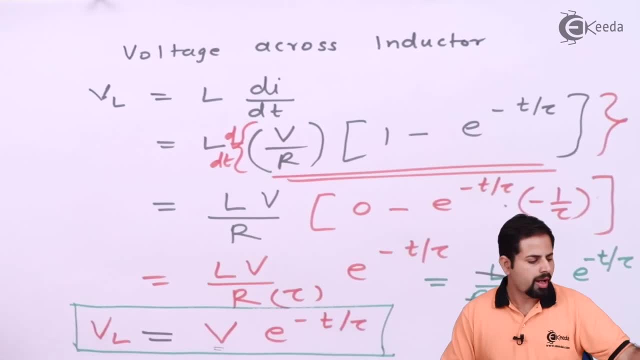 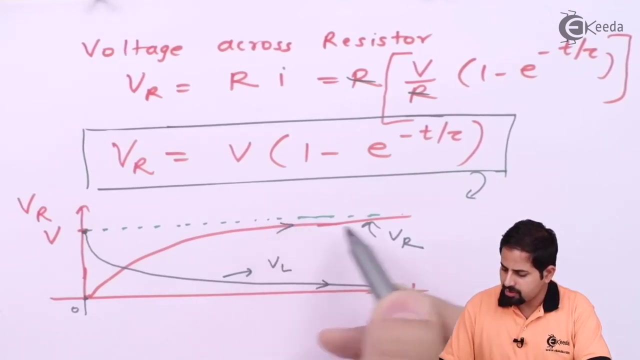 becomes 5 times tau, it will become e to the power minus 5, and you can see minus 5 is nothing but 6.73 into 10 to the power minus 3. so it is very small, and so the graph will tend to 0.. So this is how it will be, whereas resistance graph is going- was going like this: This was: 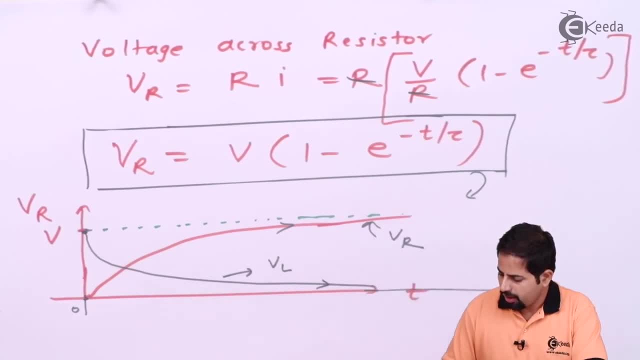 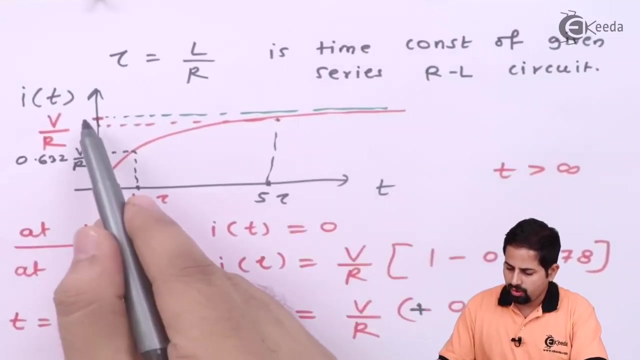 voltage across resistor and this is voltage across inductor, and this is our time. So this is all about the voltages across resistor and inductor. already we have got the graph for current, which I will show to you. This is the graph for current. this is how the current varies. maximum value is V by R.